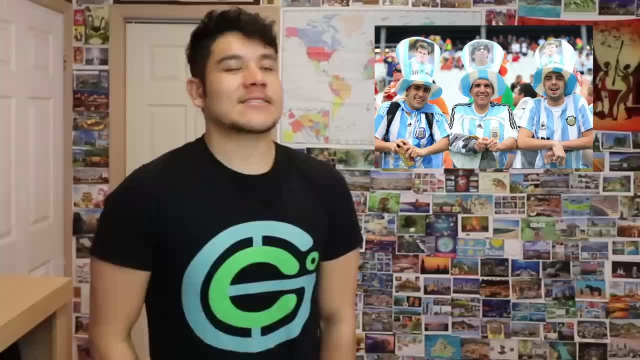 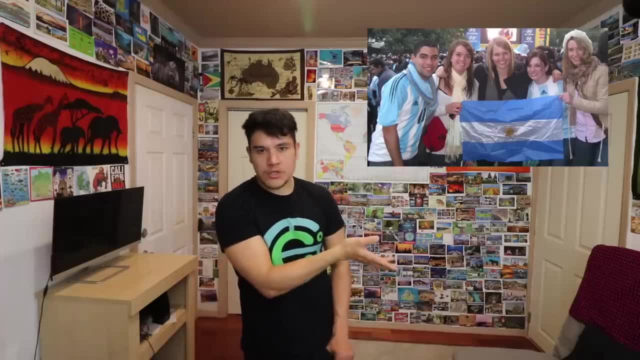 No, but in all seriousness, Argentinians are really cool, nice, sweet people, Just uh, they're kind of, uh, they're very proud of their country. Argentinians tend to be way more connected to their European roots as opposed to the other countries. 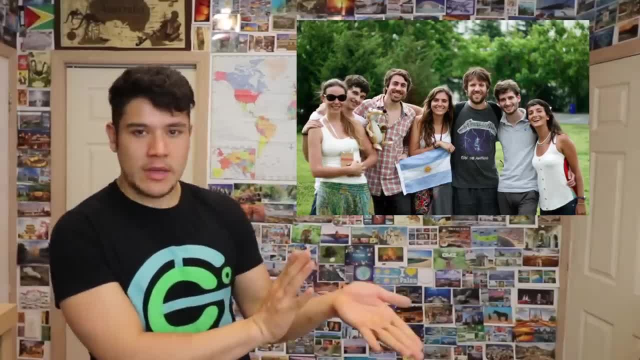 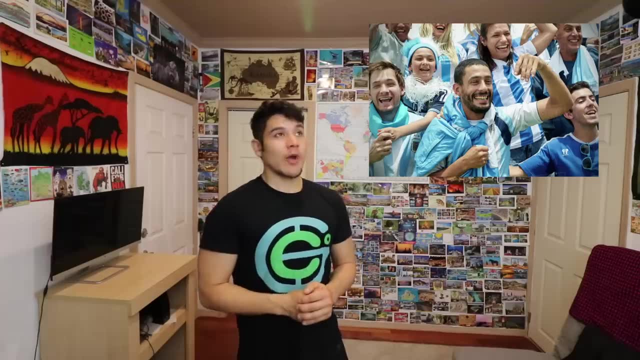 Over half the population is either Italian or has roots from Italy. You're also more likely to see blonde-haired, blue-eyed people, Of course, they are known for their passionate tango steps, Mate, And uh yeah, really cool people. 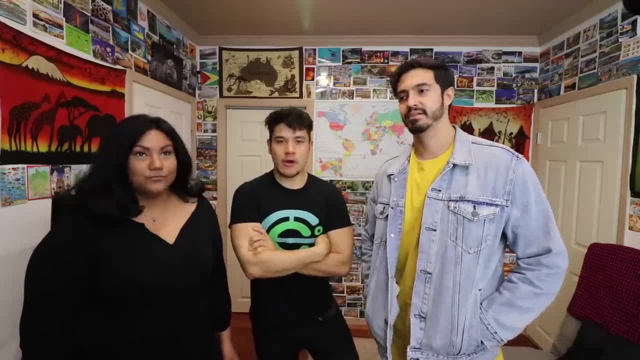 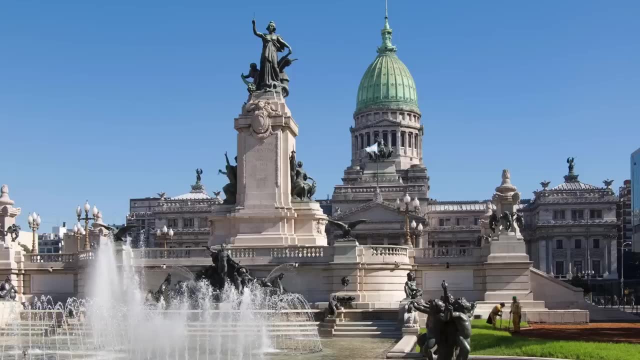 Just uh, be careful. Be careful about talking about this. All right, Cindy Diego, what do you got to say about Argentina? They have the best barbecue, like ever. They do absolutely. The city is beautiful. The architecture in the city is just amazing. 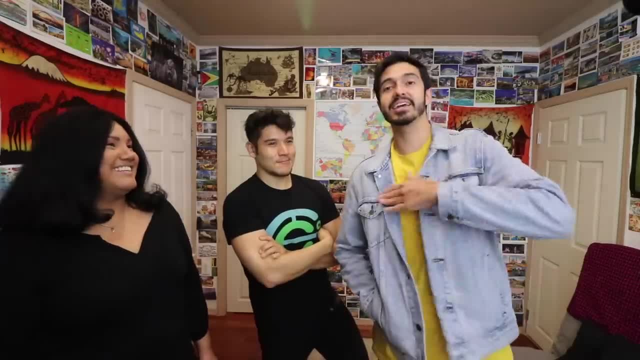 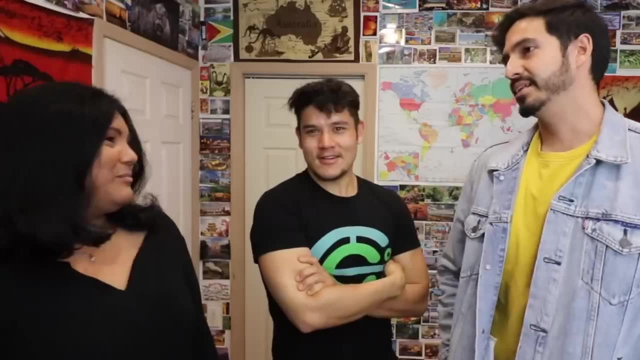 Okay. so, Diego, can you do an Argentinian accent? I'll try. Hey guys, don't judge me Please. I'll try my best. There's a lot of shh shh sounds Bolivia. Now, this is a unique one. 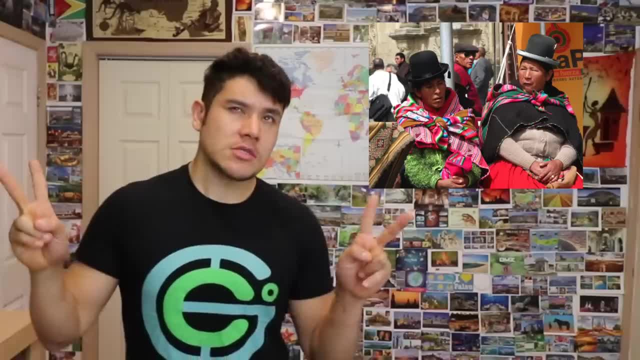 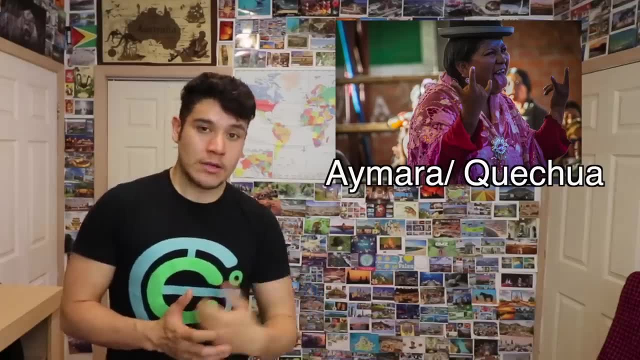 I've actually been here. Bolivia is kind of known for being like the indigenous one. They have the highest percentage of their population being Amerindian in descent, mostly being Aymara or Quechua. They're kind of like the mysterious mountain cousins that dress differently at family reunions. 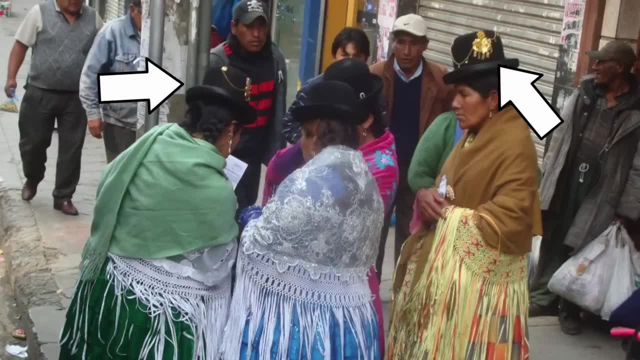 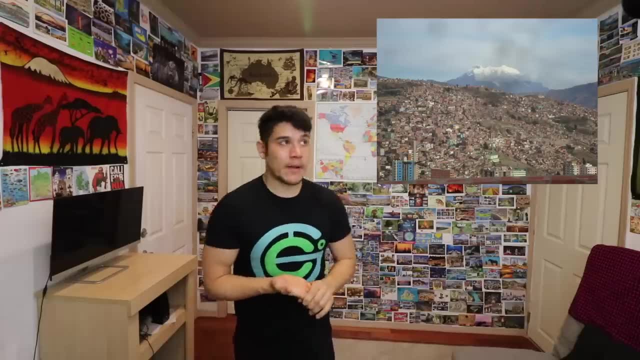 Many of the women still wear the traditional dresses and the bowler hats and wrestle. Seriously, you gotta see Cholita wrestling if you ever go to La Paz. It's like the coolest thing ever. Speaking of which, La Paz is disputably the highest capital city in the world. 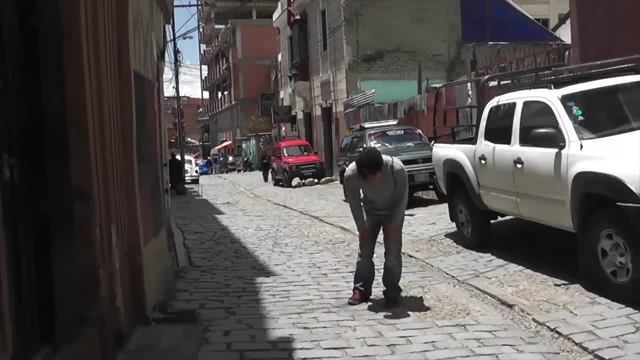 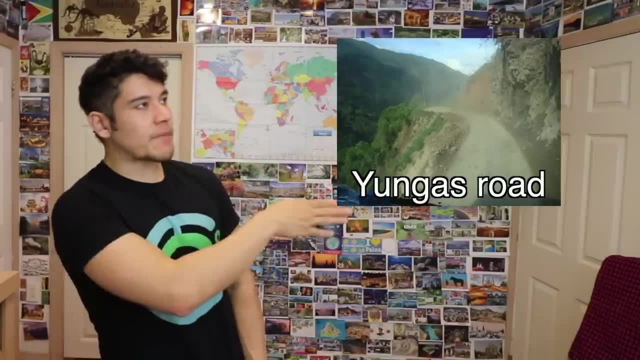 If you go there, you're gonna like run out of breath, because the altitude is so high. Keep in mind, though, Bolivia also has parts of the Amazon rainforest, and they also have a desert in the Atacama. If you go to the rainforest, though, you can pass through the Yungas Road. 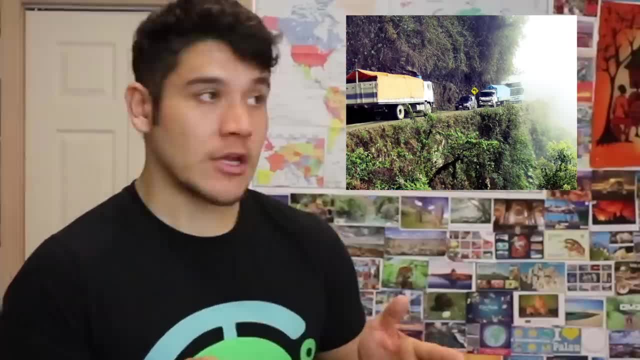 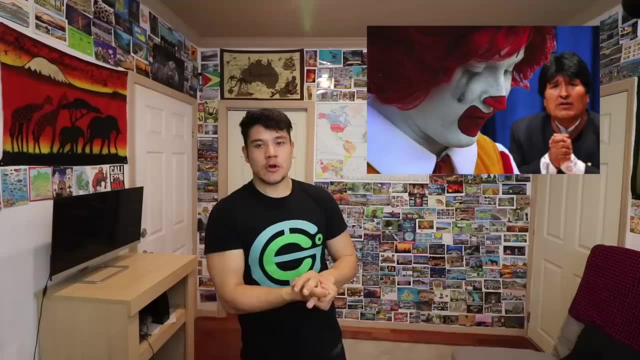 the world's most dangerous road. Sometimes it's only three meters wide. You could die So fun. They're kind of known for having a government that's like really kind of anti-outside influence. You know, all the McDonald's were banned there. 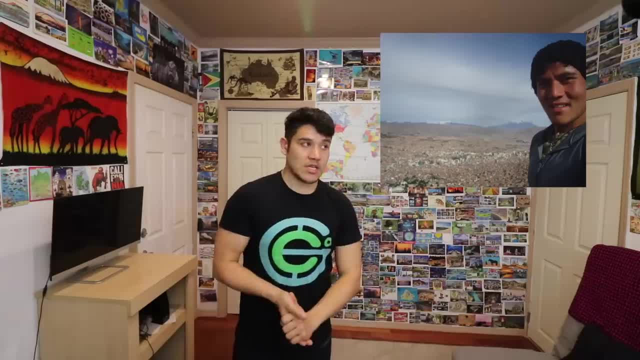 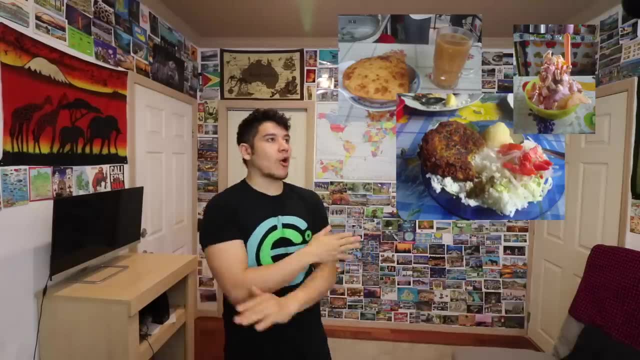 although they do have KFC and Subway and Starbucks. Oh, and because it is the lowest GDP per capita country in all of South America. the exchange rate is amazing. Not even joking, you can buy like a whole meal for 80 cents. 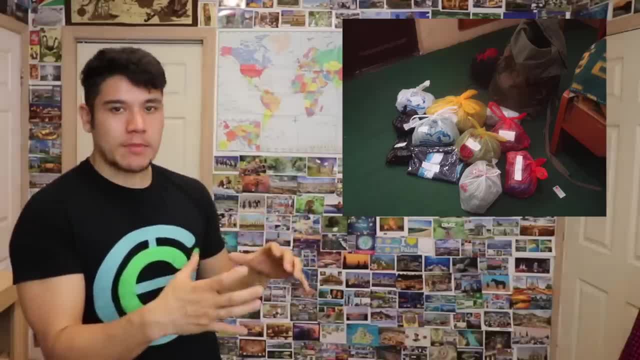 I bought an entire like army sack of souvenirs for like 20 people. I ended up spending only like $80.. Anyway, Bolivia, cool place, Check it out. All right, guys. what do you think about Bolivia? 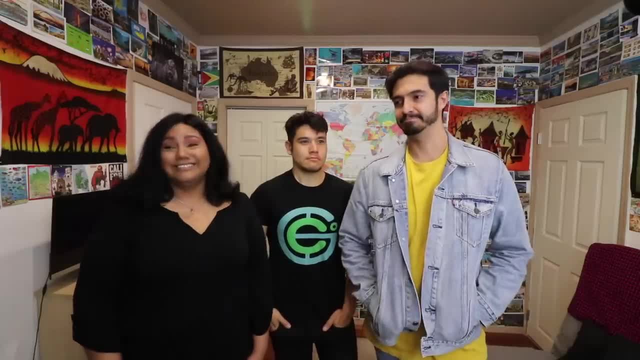 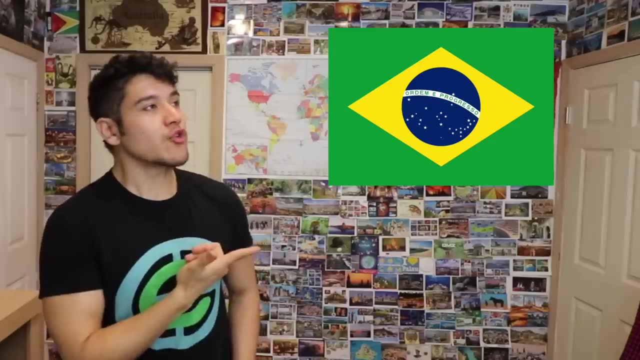 Did you caca? Uh yeah and uh. Sorry guys, No, the Bolivian people I've met. they're pretty cool, They're so down-to-earth. Brazil- I feel like I don't even really have to say too much about this. 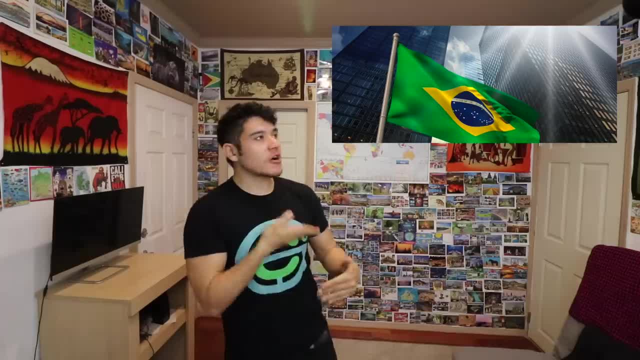 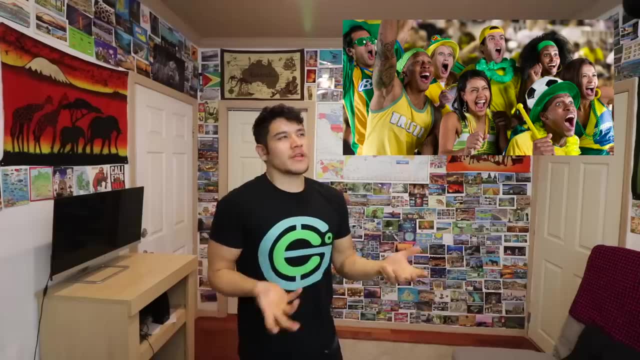 but you guys all know Brazil, It's the big guy. It's the largest country, the largest population, the largest economy in all of South America. South America could not function without Brazil. Now there's really no one way to summarize all of Brazil. 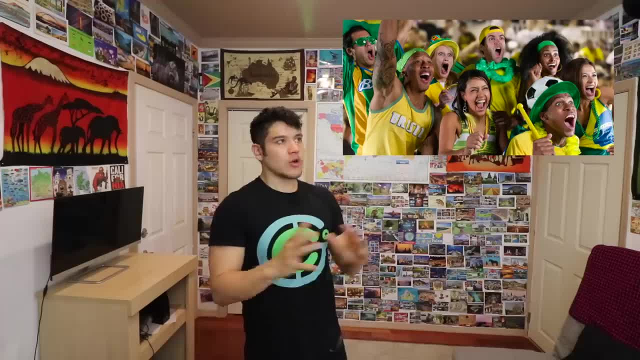 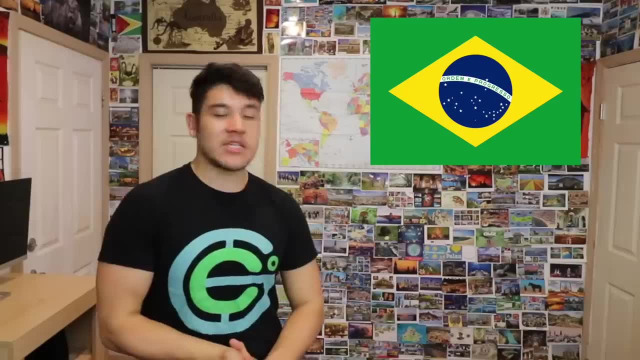 because all the regions and states are so completely different, so many different types of people. but overall it's kind of like the dad of South America, Like it plays such a key figure role and it speaks Portuguese. Brazilian Geograpeep Nadia says: 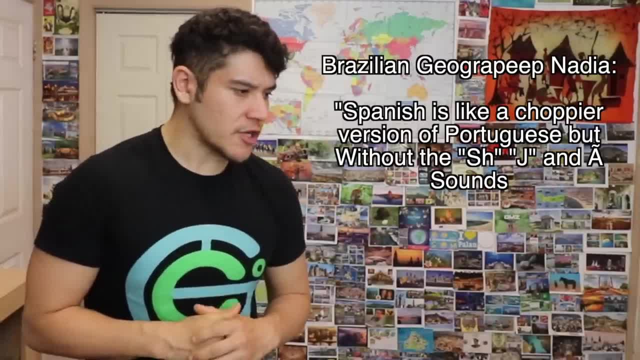 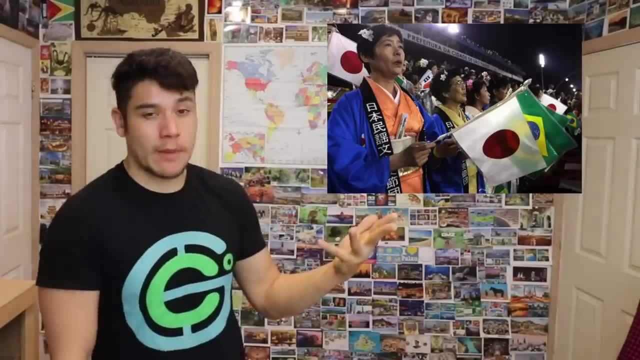 Spanish is like a choppier version of Portuguese, but without the sh, j and n sounds. The country is super diverse. You have white, black, Asian. They have the highest Japanese population outside of Japan, And it's interesting, though, because it doesn't matter who you are. 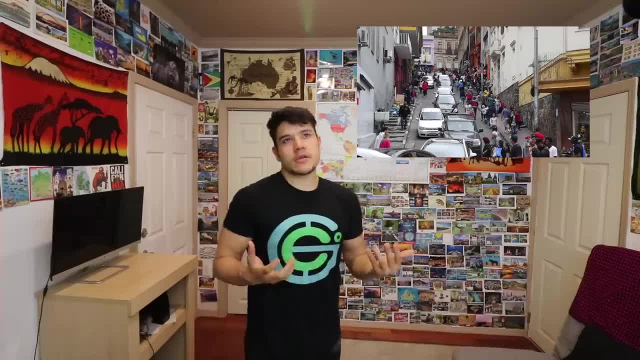 Like at the core of their hearts. they're Brazilian first. I mean Brazilians. they know how to get down to it and work really hard if they have to, but I mean when you're surrounded by so much natural beauty. 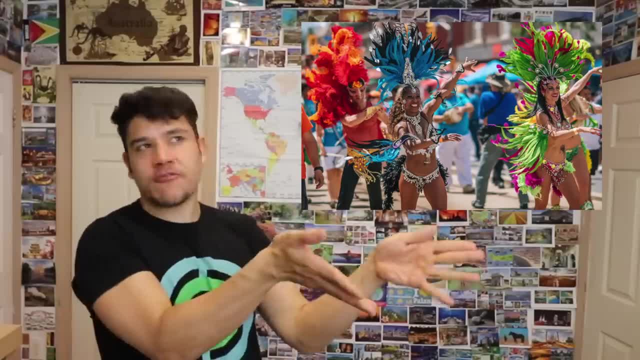 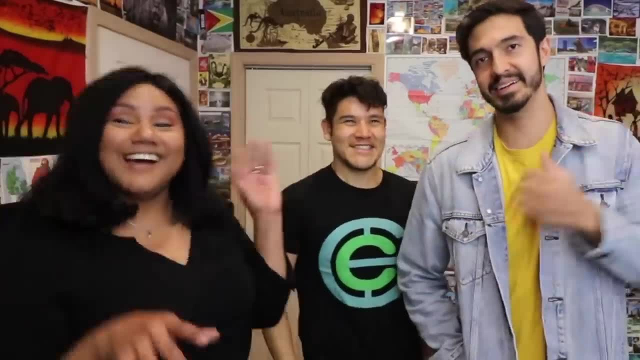 it's really hard not to relinquish the samba from your soul. And that's kind of Brazil. you know Brazil. what comes to mind? Brazil? I love their people. They're super cool. Like you just want to party with them. 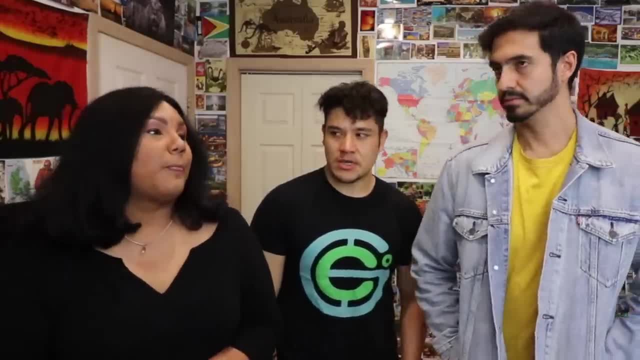 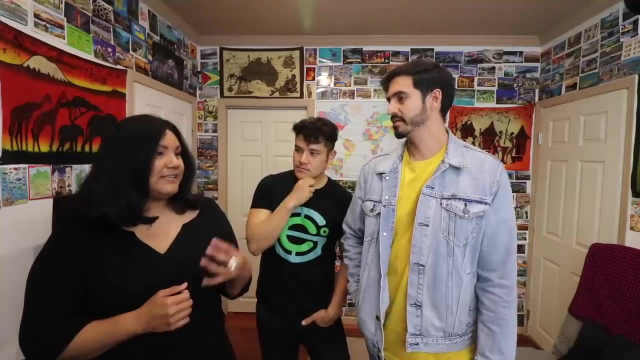 What do you? How much Portuguese can you guys understand when they speak it? I mean, I would say I would get like 20%, 30%, Even 40%, Maybe even 40%. Yeah, I feel like it's like a Spanish with an accent. 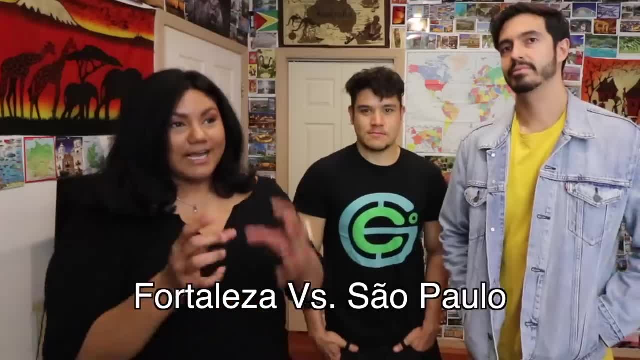 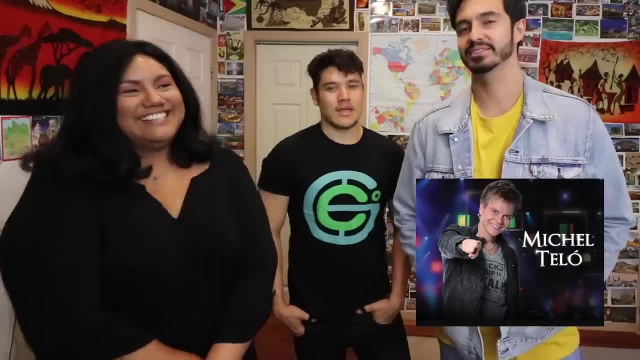 Yeah, it depends, And also depends the region, Because for the list it has a heavier accent. Sao Paulo not so much. I see what's in my eyes. I gotta look this up. Chile: This one's interesting because geographically speaking, 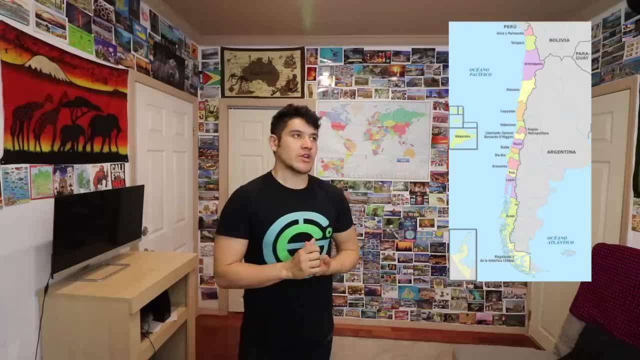 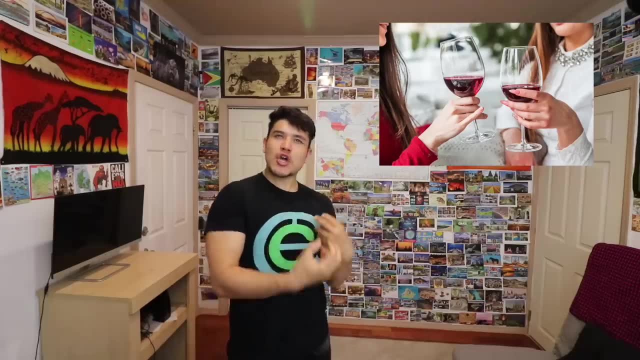 they are pretty isolated from the rest of the continent. It's like the only country in the world where you cannot do a horizontal landscape layout of the nation's image. Chileans are kind of like the bougie stoic, Ralph Waldo Emerson- writers who drink wine. 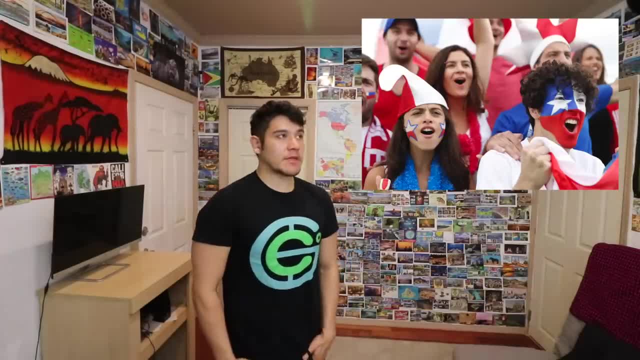 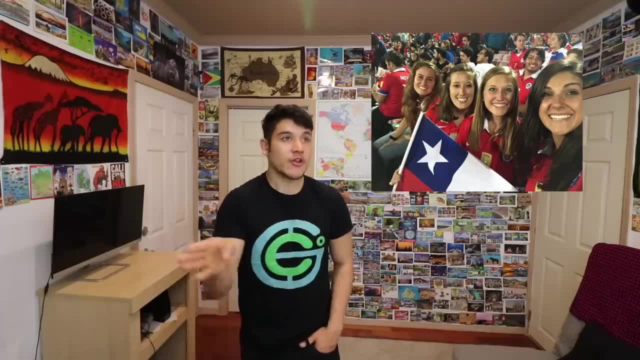 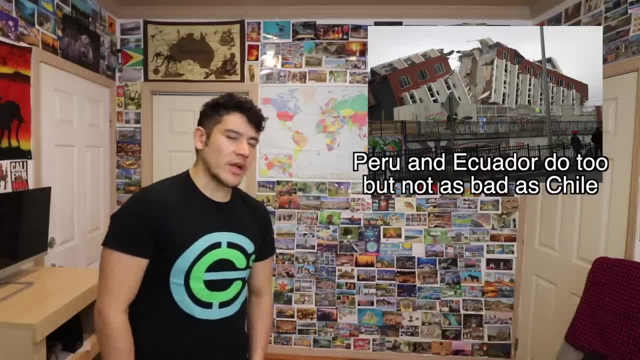 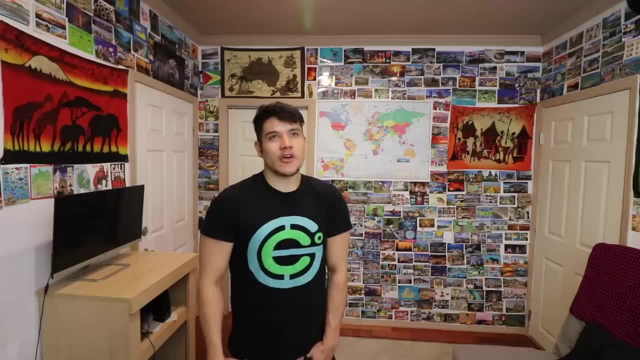 That's how thick their accent is And it's interesting because they're kind of like the only country that really has to deal with intense earthquakes. They are right on the Pacific Rim and they get a lot of penguins, But overall, yeah, it's like they're kind of like the 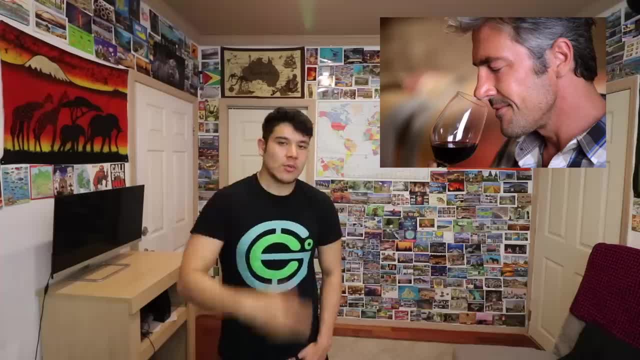 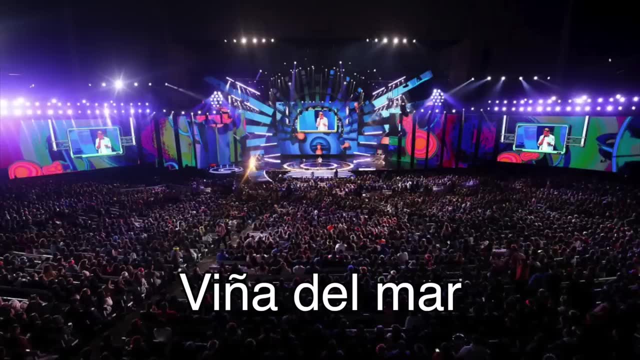 slightly rich uncle with a pipe in his hand, but you just can't understand what he's saying. Chile: what comes to mind? Pololos, Pololos, And they're famous for their festival, that they have Viña del Mar. 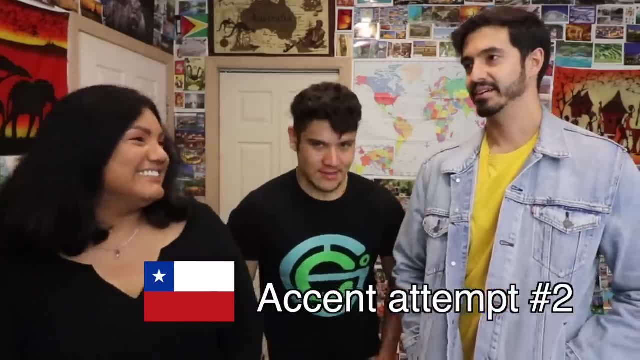 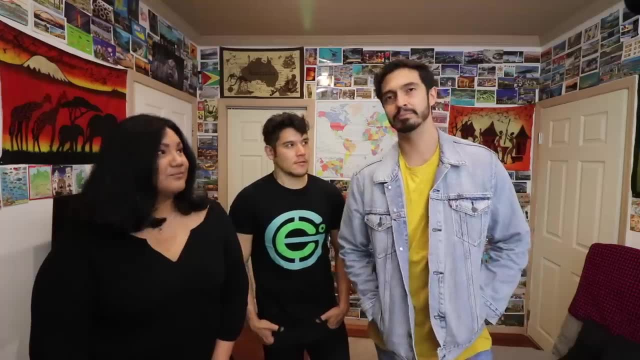 Yeah, it's really nice. Diego, can you do a Chilean accent? Sorry, guys, that sounds so stereotypical, My bad. Is there such a thing as pololear in Chile? I don't know, Like to make a boyfriend or girlfriend. 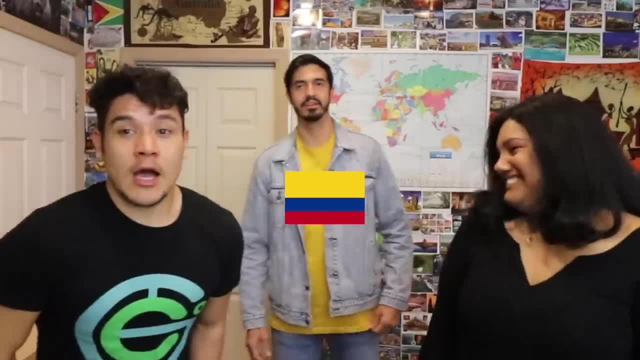 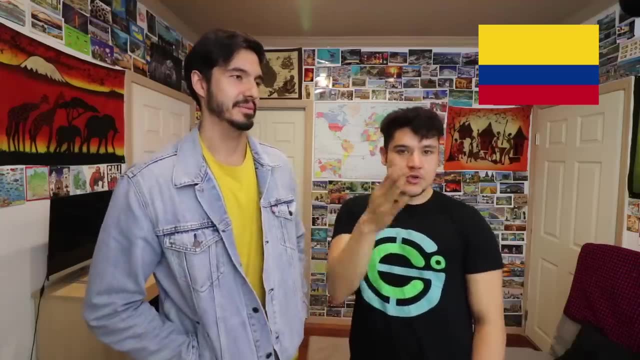 Like a verb. Any comments Maybe, But let us know. And now Colombia. Diego's time to shine. Cindy, you're gonna have to sit this one out for a little bit. All right, South America was a family. How would Colombia fit into it? 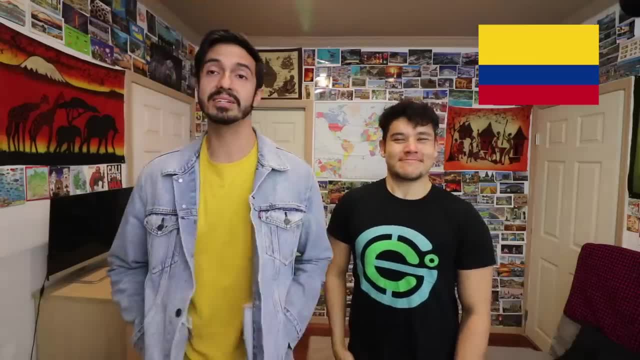 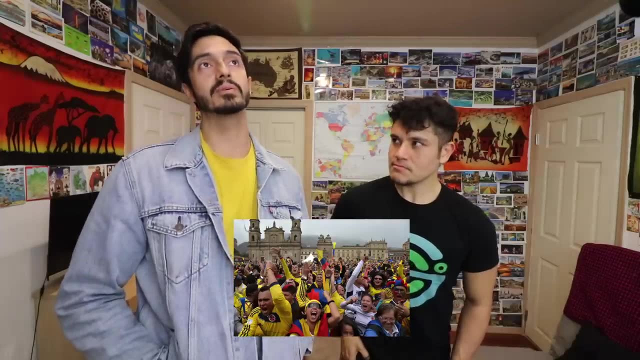 They said we're the troublemakers. but let me be clear: Party-wise, yes, we are the troublemakers. party-wise, Party, Yeah. First of all, we're a country that you know we don't give up, like against or like with. 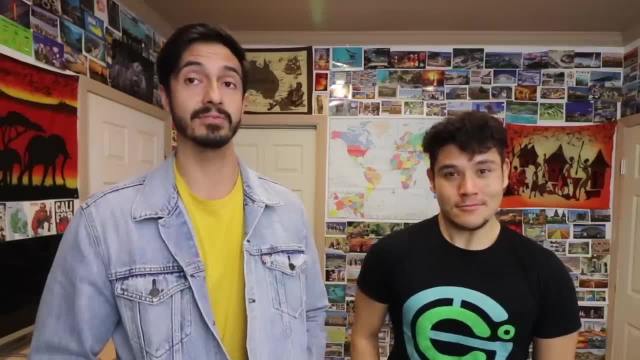 adversity like facing adversity. You had a lot of it. Yeah, we've been. we've gone through a lot. It's interesting, You guys are kind of like the twin of Venezuela, right. You're like very similar, right. 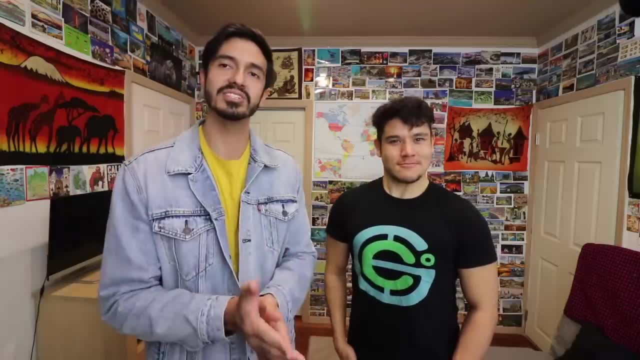 Yeah, It's funny because we're like we have this like love and hate relationship. Yeah, In the 80s and 90s, Colombians were going to Venezuela. Yeah, They were running away and going. Now it's the opposite. 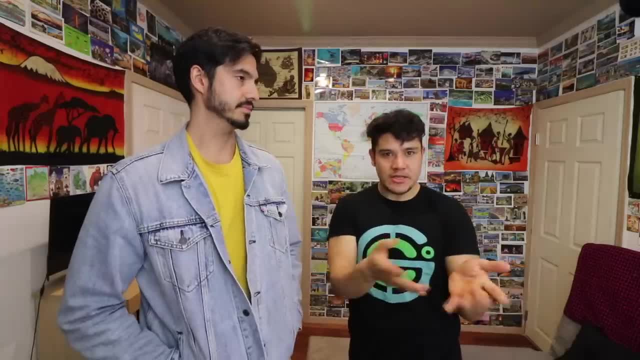 Venezuelans are coming to Colombia. You're right. There is like a unity between you guys: Yeah, No matter what happens Exactly, You're always going to be there for each other, And Colombia has taken the most Venezuelans out of any other country in the world. 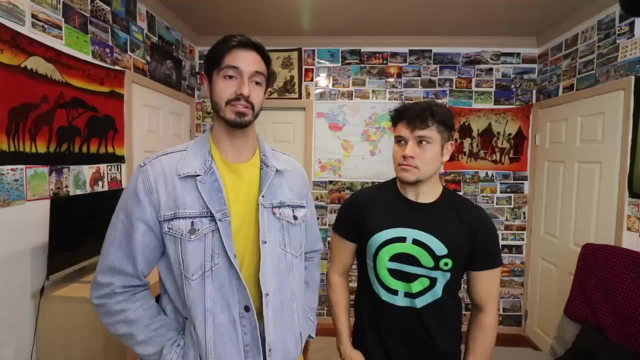 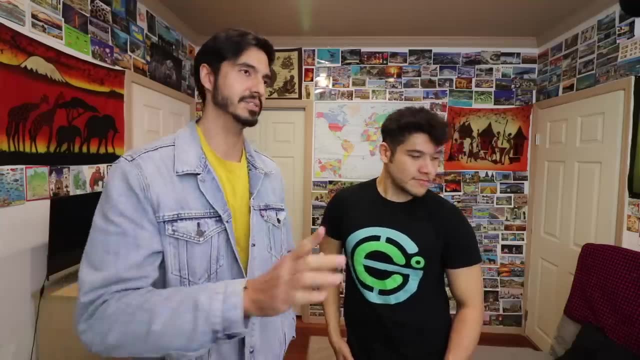 Yeah, I heard it's like you know it surpassed like the million. I mean there's a lot of great food, great music, beautiful girls, beautiful women And, by the way, guys, we have the original arepas. 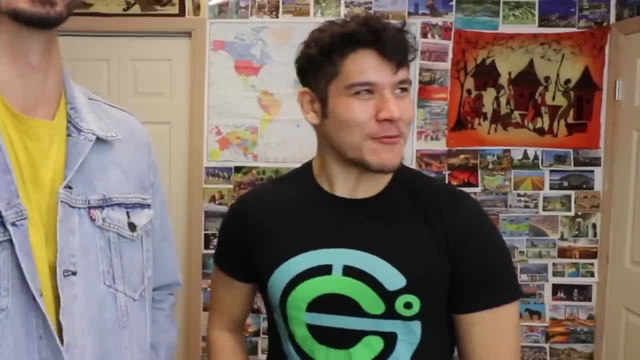 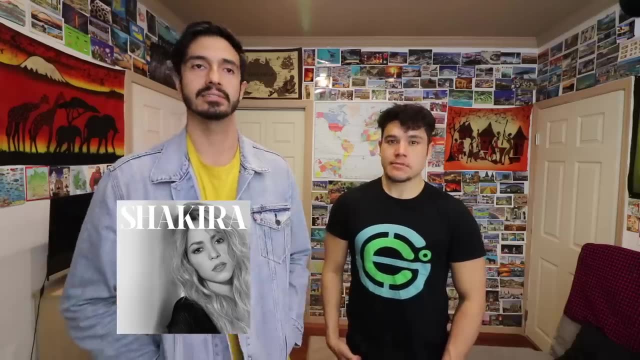 So it's all good, Venezuelans are going to argue about that. Yeah, So many musicians and artists, right? Yeah, For example, J Balvin. you know he's been killing it. You know Shakira Juan is. 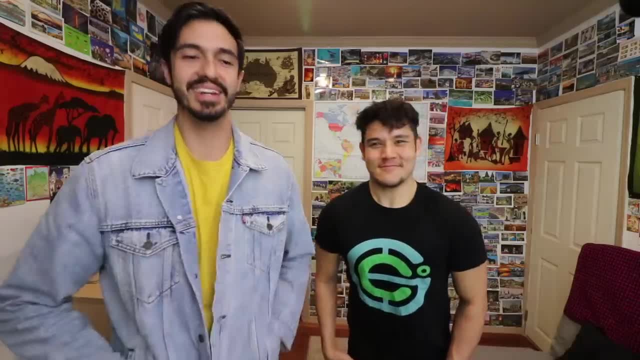 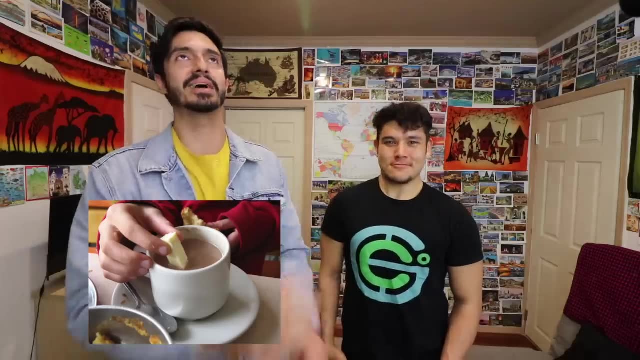 Everybody knows Shakira, And the list goes on. I mean I don't know if it's weird to you guys, but like we love to dip, like cheese queso cojado or queso campesino- like into hot chocolate and it melts and it's the best. 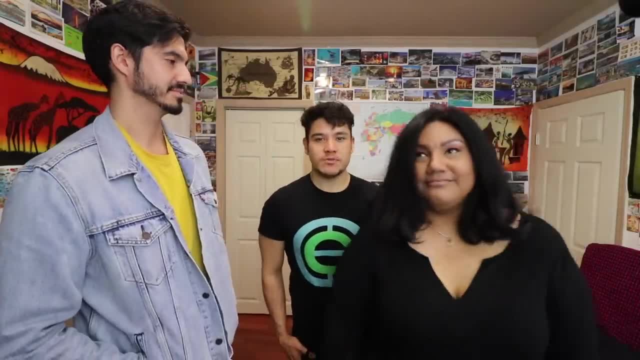 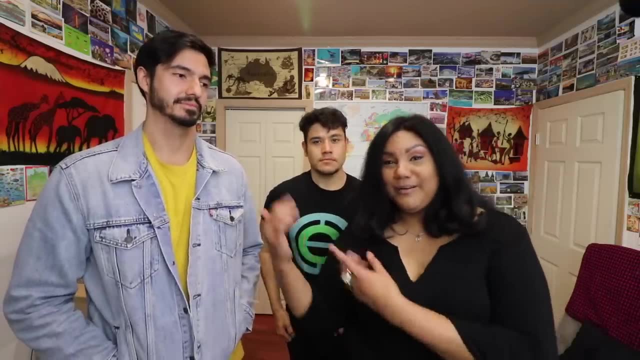 thing ever. All right. Well, Cindy, what is an Ecuadorian's perspective on Colombians? Yeah, the chocolate actually was pretty good. I can say that I really liked it And they're pretty cool people. I mean, don't you see this? 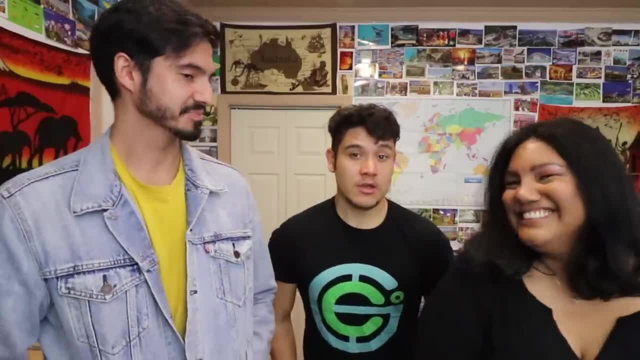 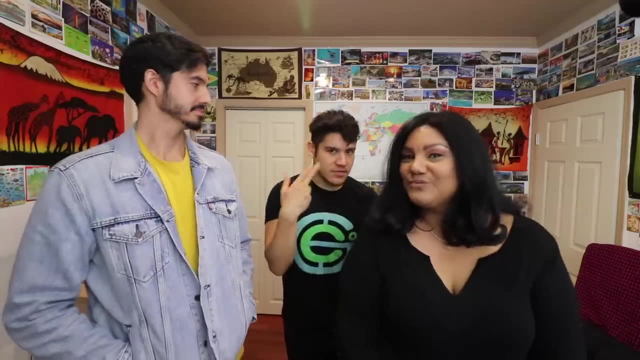 I mean, it's like, yeah, they're pretty awesome. And it's interesting to note that also these countries, as well as Venezuela and Panama, were one country at one point- Yes, Gran Colombia. So you're going to see a lot of similarities and you know cultural traits, that kind of. 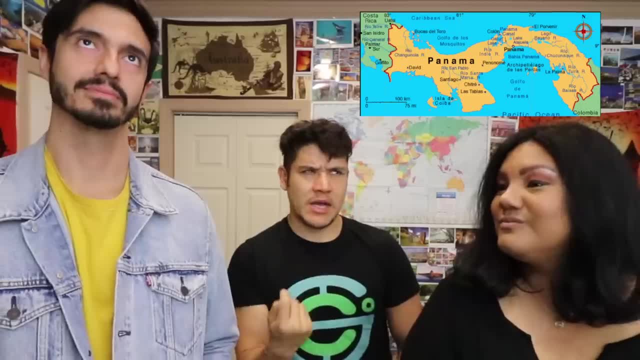 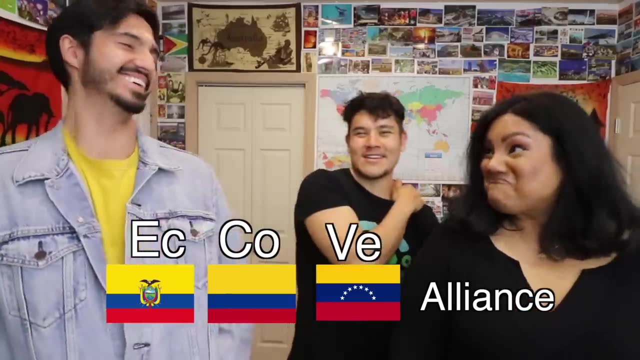 tie in with each other within all four of those countries- Maybe less Panama, though, because they're kind of a little separated- But Colombia, Venezuela, Ecuador- I call it the ECOVEY Alliance- And now Ecuador, which means Diego, you got to get out of here. 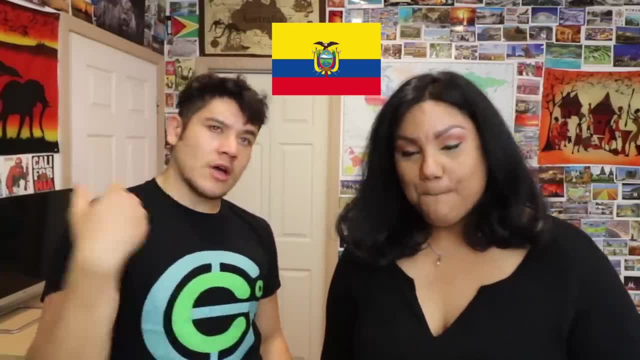 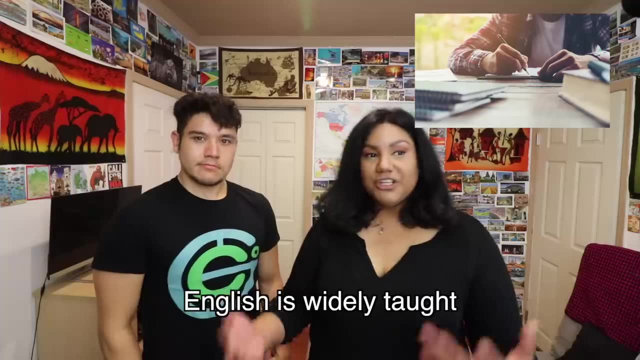 All right, Cindy, if South America was like a family, how would Ecuador play into the mix? I don't know. Ecuador is very chill. We're very nerdy. We do love education. Like all our schools are bilingual. Like everything is focused in education. 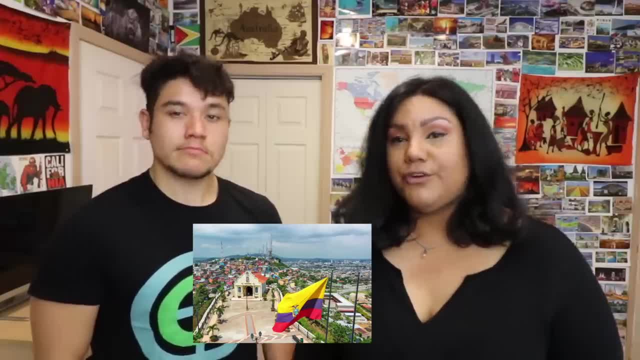 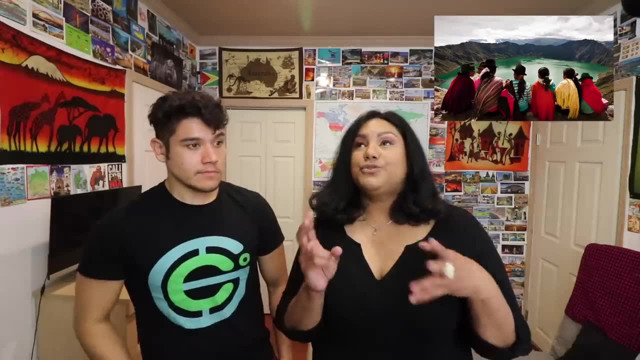 We are a very friendly country. We don't like to fight Very agricultural, Kind of like the sidekick best friend. I would say totally that Yes, The second language was official. The Quechua language was in 2010,, if I'm not wrong. 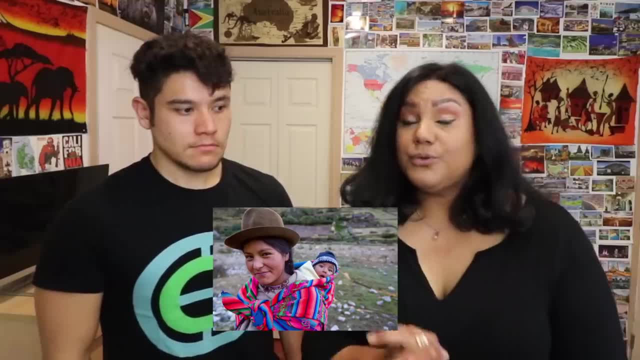 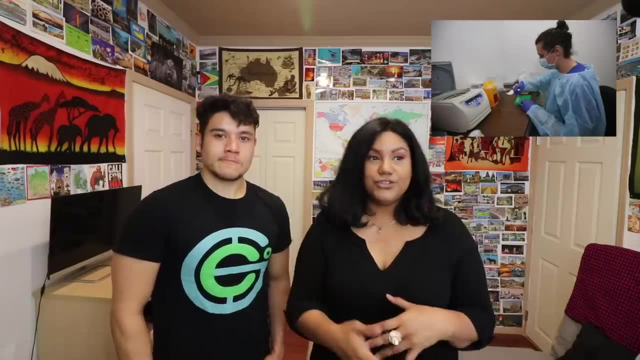 They made it official. They made it official in our country, But, yeah, and now a lot of schools are actually teaching Quechua And the Darwin Center is actually in the Galapagos. So there's a lot of research, There's a lot of you know. 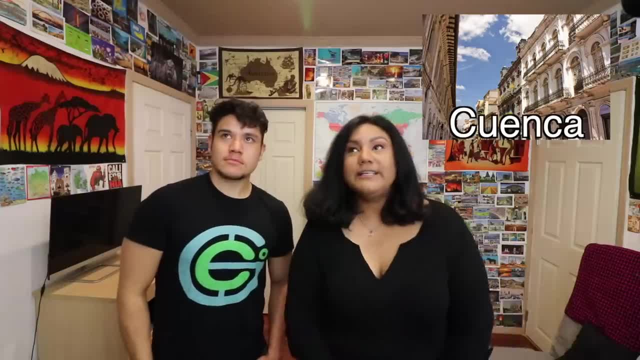 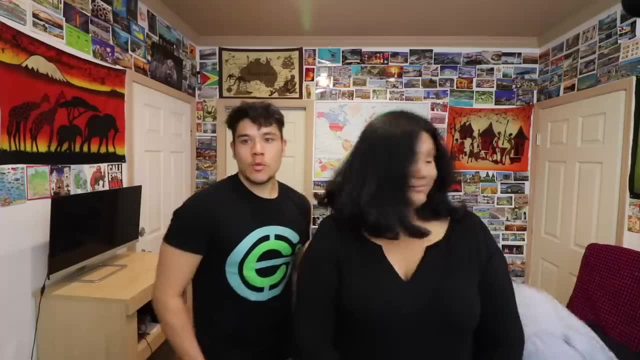 A lot of science-y stuff. A lot of science-y stuff. Yeah, Okay, so Cuenca is a very colonial place. It has become like the number one retirement place in South America. Well, Diego, from a Colombian perspective, what do you guys think of Ecuadorians? 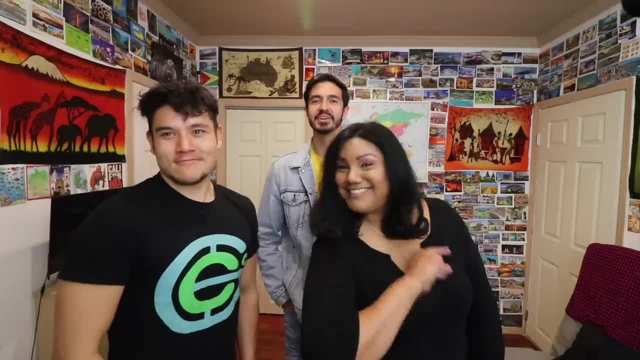 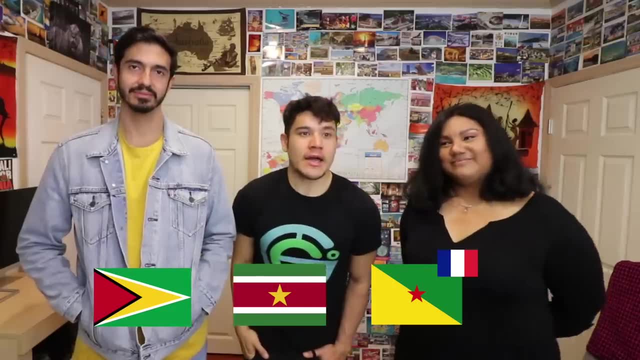 I think they're pretty chill. you know, We never had a problem with them. They're kind of like the nerdy brother, you know who like never messes, you know with you. so All right, guys, what do you think about the Guayanas and Guiana and Suriname? 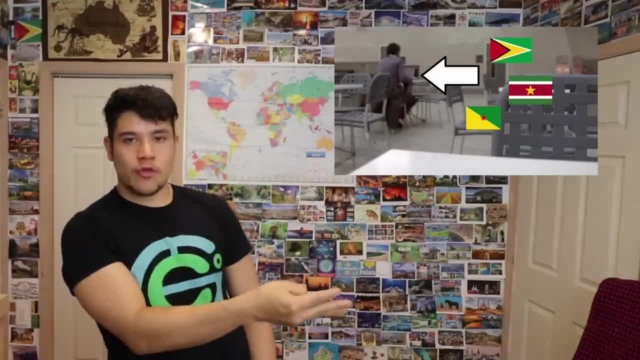 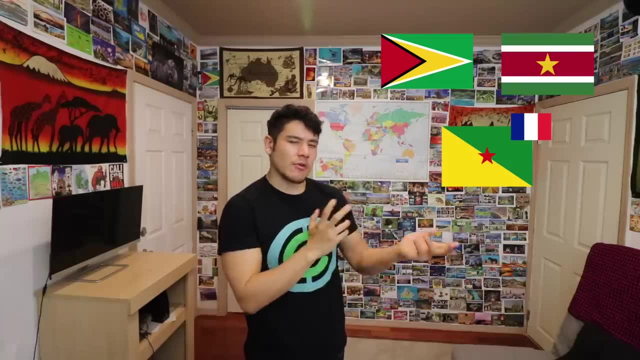 Basically, these three are like the quiet kids down the hall at school that you didn't even know went to your school and, like you, meet them for the first time at graduation. Now for Guiana, Suriname and French Guiana. I'm just going to kind of do them all at once. 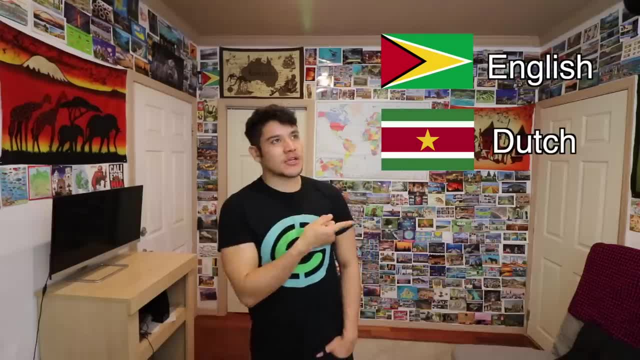 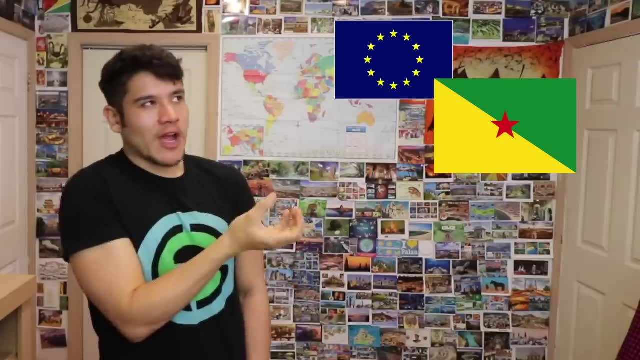 because these three just kind of generally go together. Guiana speaks English, Suriname speaks Dutch- although English is very prevalent there as well- And French speaking French. Guiana is an overseas region of France, which is why some people kind of use it as like a backdoor entrance into the EU. 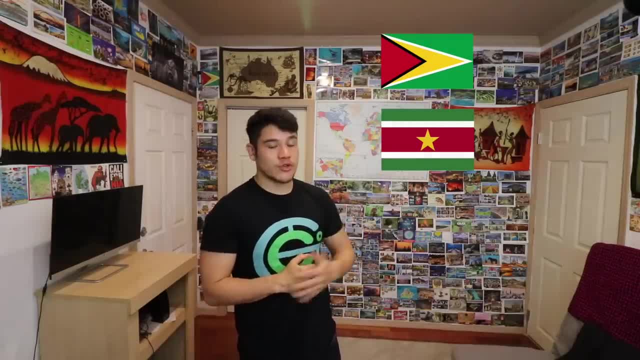 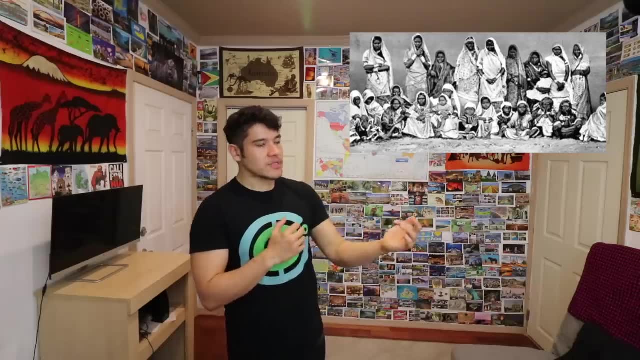 Otherwise, yeah, Guiana and Suriname are also very similar. They're the only two countries in South America that draw on the left side of the road. They both have huge Indian populations, people that are descended from the indentured servants that were brought over during colonial times. 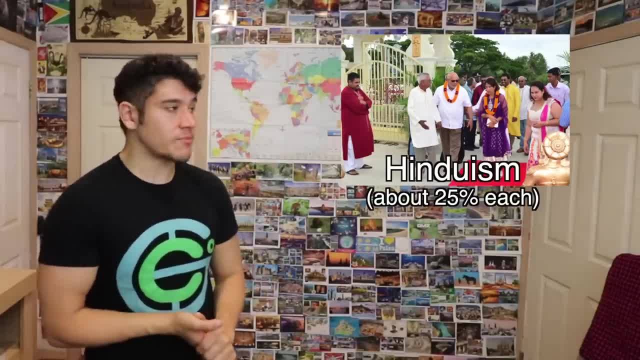 This, in return, makes them some of the countries with the highest Hindu populations per capita. You can see Hindu shrines and Hindu temples all over. Basically, in a nutshell, it's kind of like a place where a ton of different people from. 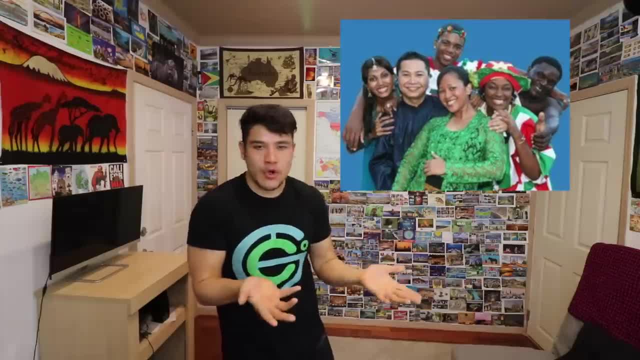 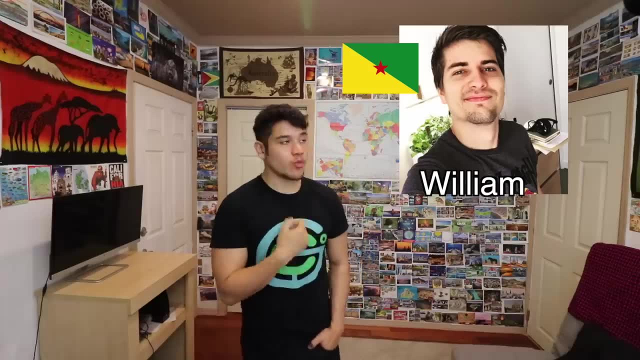 all over the world were dumped into one spot and had to kind of figure out what to do. These three areas generally identify as Caribbean in their culture and identity, rather than South American. I talked to my French friend, William, who was born here. 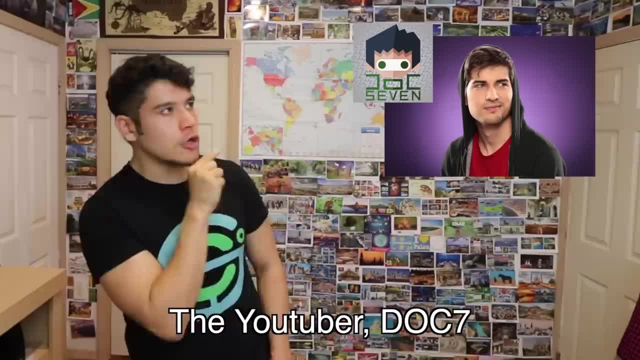 Certains d'entre vous peut-être le connaissent, The YouTuber Doc7.. Yeah, we're buddies. He was actually supposed to be in my France episode but you know, life stuff happened and he couldn't make it. 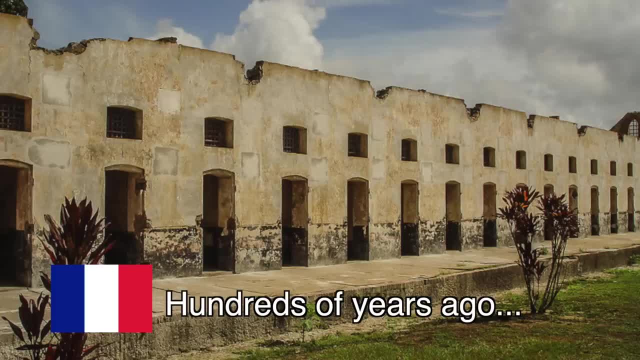 But yeah, we still keep in contact. Anyway, Doc7 wanted me to tell you French Guiana was started out as a prison colony where some of the worst criminals in France were sent, similar to what the British did to Australia. It's super diverse. 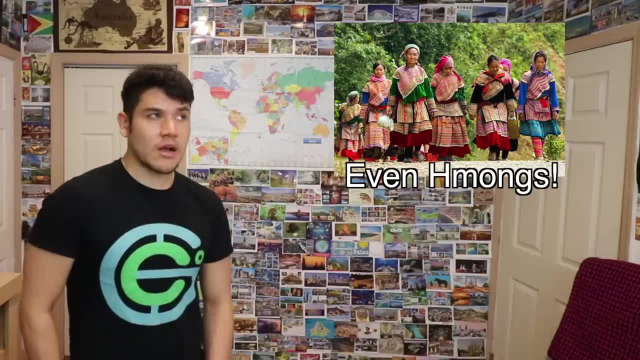 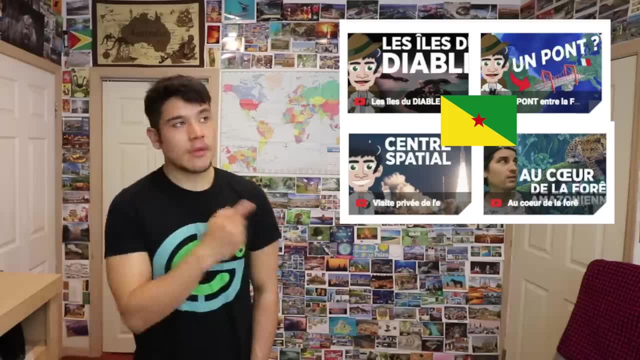 They have whites, blacks, creoles, native Indian tribes. Surprisingly, a lot of Hmong people that were brought over after Lao had a big war. They're famous for their space center, the Chute Voltaire. He actually made quite a few videos explaining about this place. 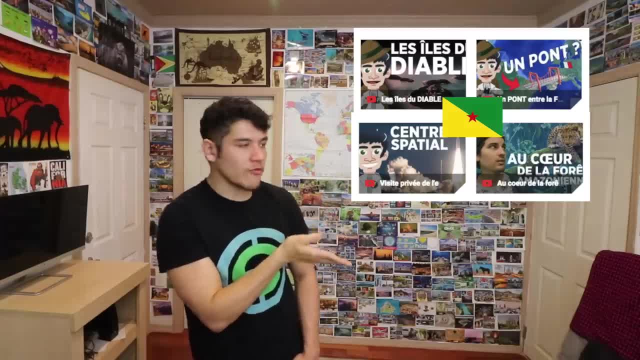 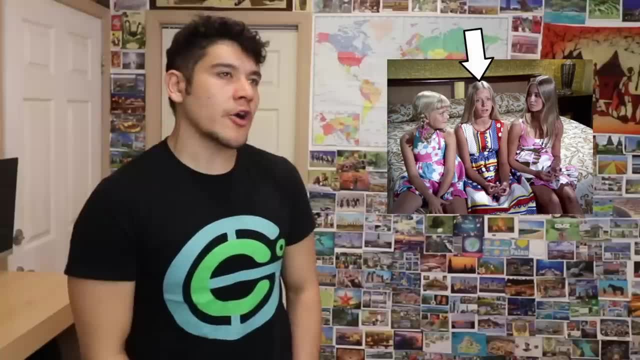 Most of his videos are in French, but some of them do have English subtitles though. So if you don't understand French, just turn on the subtitles. Paraguay- Paraguay is kind of like the middle black sheep daughter. that doesn't get a lot of attention. 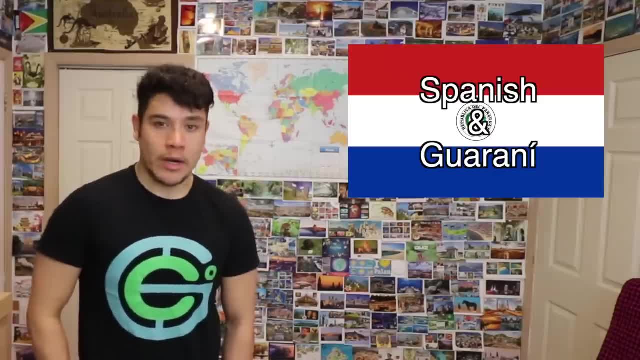 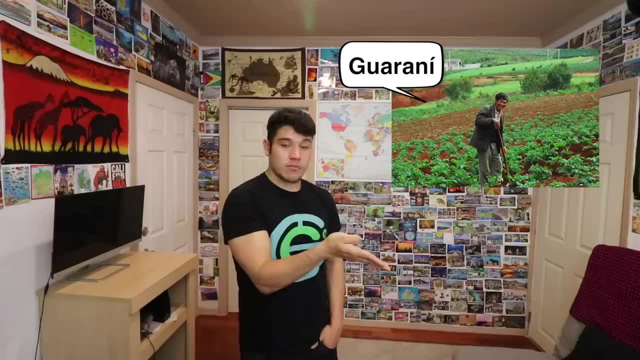 Paraguay has two official languages, Spanish and the indigenous Guaraní language, And it's interesting because more people actually understand Guaraní than Spanish here. If you go outside of the cities into, like rural areas, you might even have trouble communicating because the people just don't speak Spanish. 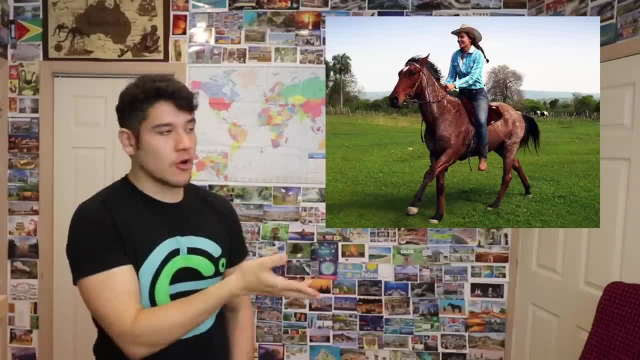 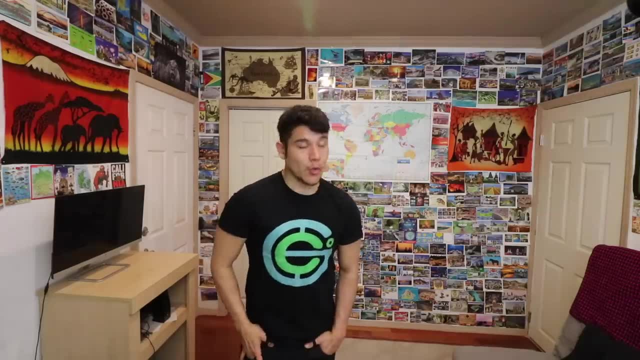 But naturally they are kind of like more rural and rustic. They're known for being good horse riders, They love drinking tereré, They love playing that bouncy galopas and guarinas country music And finally, the women are famous for doing the danza de la botella, or the bottle dance. 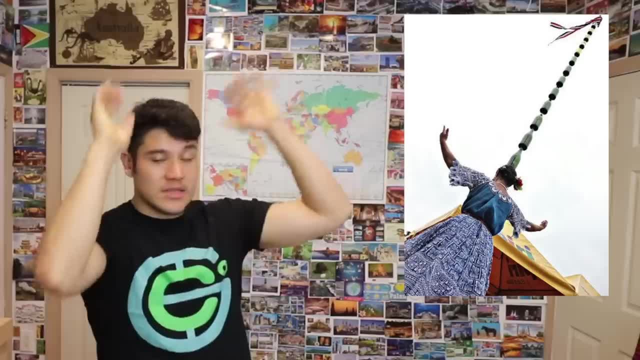 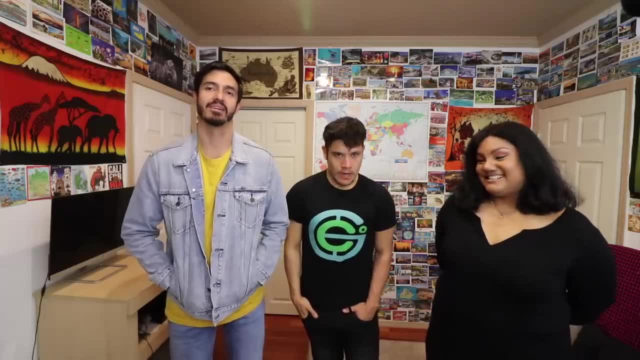 It looks really cool Like they balance bottles or jars on their head And sometimes they stack them up like 10 high. Pretty cool, Very underrated. I say: go visit All right guys. So what comes to mind when you think of Paraguay? 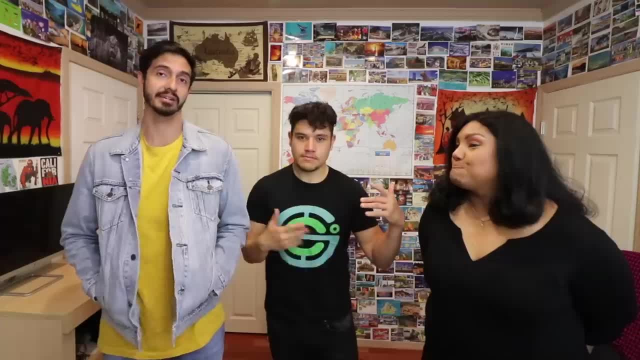 If I'm not mistaken, they're pretty good with like playing harp Harps. I don't know, maybe What kind of comes to mind when you like meet or like see Paraguayan people on TV, or what do you think? 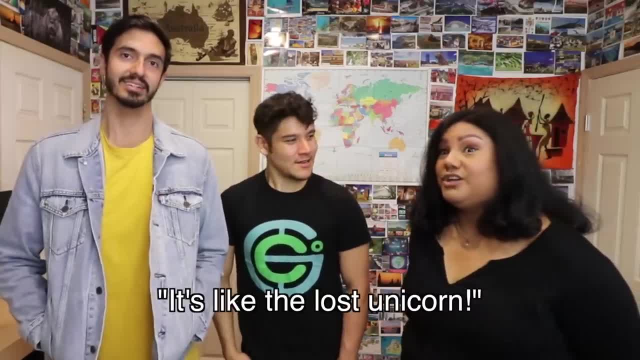 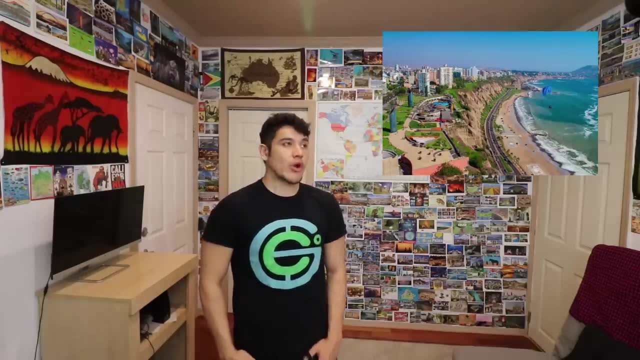 Or how have you guys been all this time? I know It's like the lost unicorn. It's a mystery, Peru. Peru is kind of like the big brother who took a risk, played his cards right in business and marketing and exploited the crap out of all his tourism spots and made a lot of. 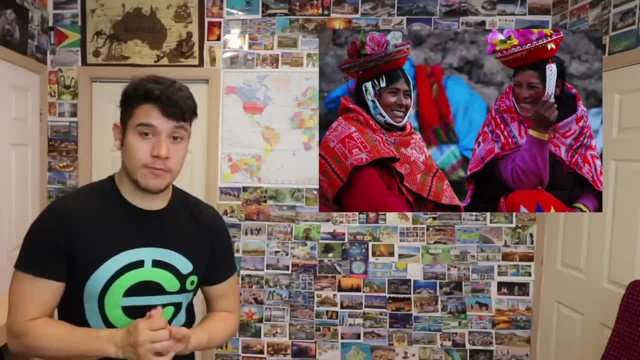 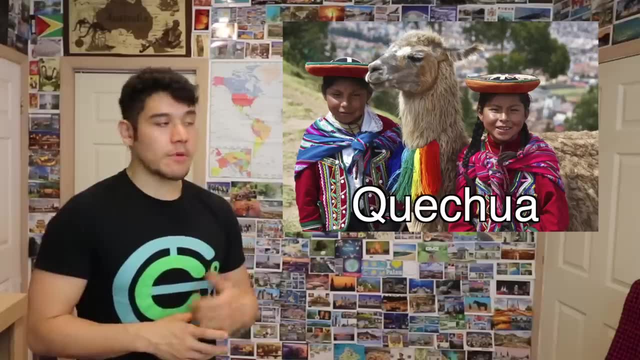 money. It worked. He's kind of like a big shot now. Keep in mind, Peru is also one of the indigenous strong nations. A significant portion of their population is Amerindian in descent, Largest one being Quechua. They are known for having really good food. 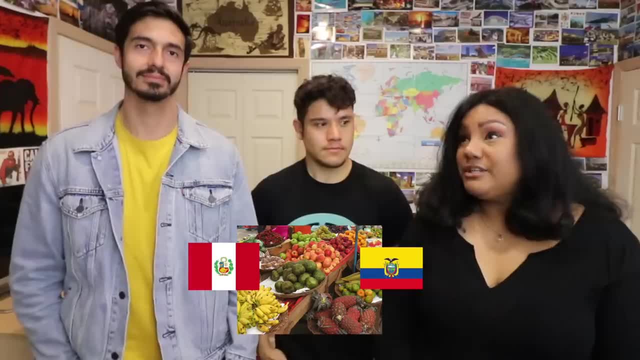 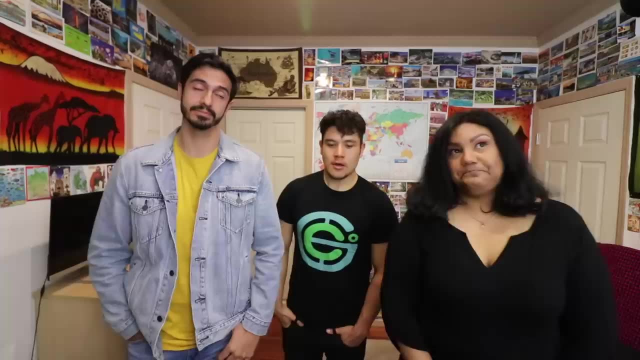 Everybody knows ceviche. All right guys. Peru- What comes to mind, Particularly Ecuadorian and Peruvian food is very, very similar, Even like the papas that they have. Oh really, We have it. It is very similar. 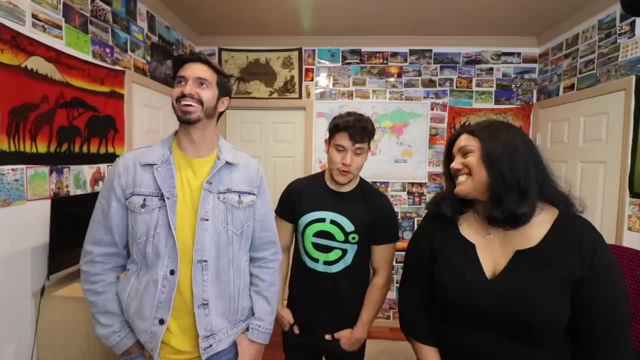 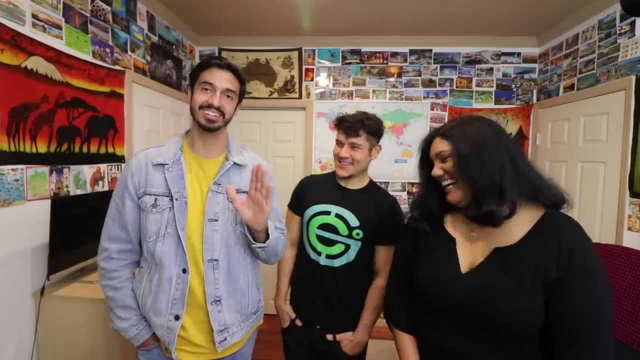 Okay, Diego introduced me to this wonderful, amazing thing from Peru. What is it, Guys, please don't hate me, Okay, But I had to. I love it. All right, You know what it is already, Señorita Laura. 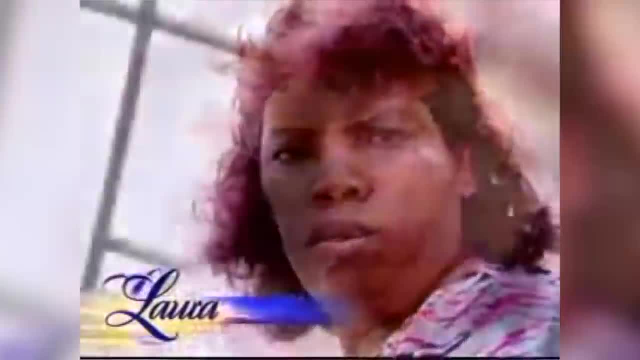 For those of you who don't know, Señorita Laura is Señorita Laura, Like the Jerry Springer of Peru. People go on this show and they go crazy and they yell at each other and they accuse who of cheating who. 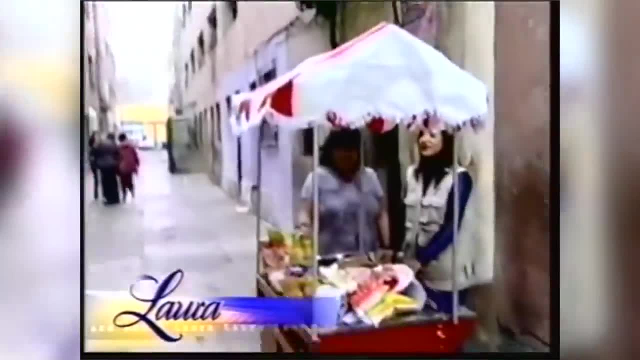 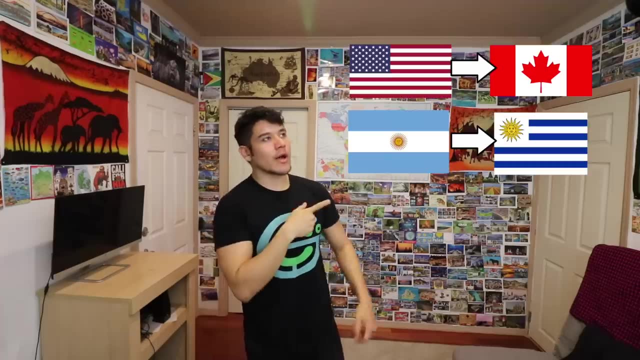 And then some of them get a prize, And apparently this lady got a hot dog stand as a prize when she was cheated on. I don't get it, but I love it, I love it. I love it so much. Uruguay: The joke is, Uruguay is like Argentina's Canada. 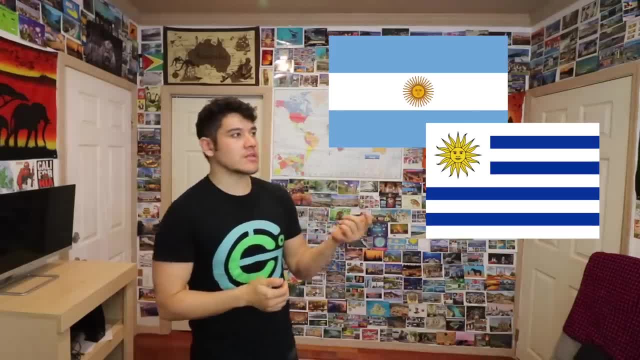 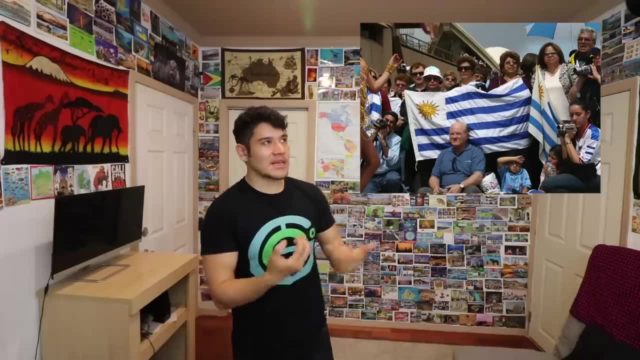 Most South Americans say that they can't distinguish the difference between Argentinians and Uruguayans. But Argentinians and Uruguayans can totally tell the difference and they swear by it. They have like generally the same accent and the same general kind of like Eurocentric type of demographic. 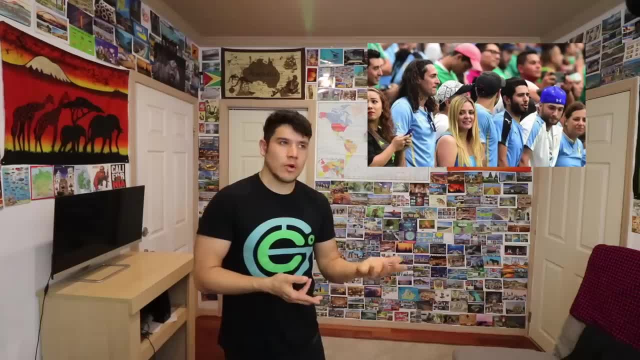 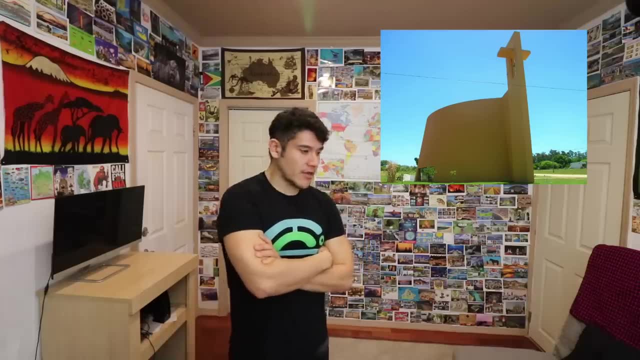 I mean Uruguay doesn't really have a native indigenous population. The ones that were there were kind of either moved or displaced or killed off, So now it's mostly just Spanish and Italian. Out of all the countries in Latin America, they have the lowest percentage of church. 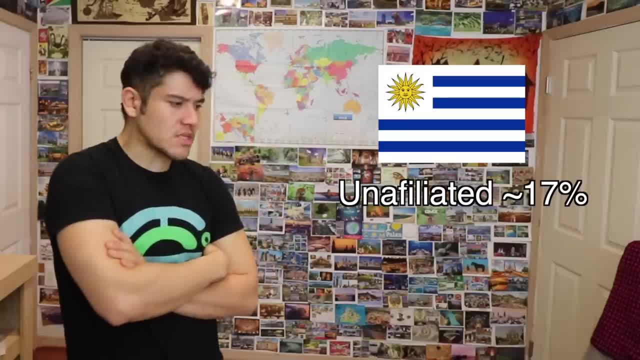 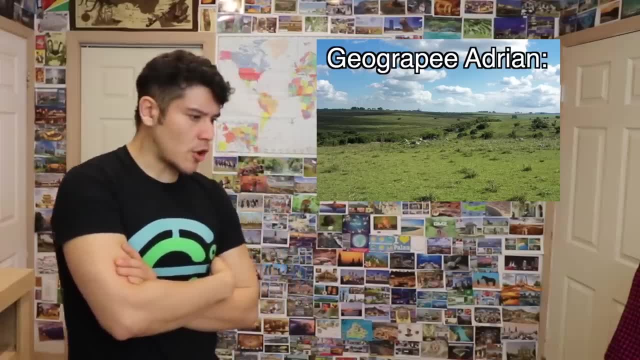 attendance and highest unaffiliated population, at somewhere around 17%. Landscape wise Geograpeep Adrian says it might be boring. We don't have mountains, deserts, jungles or snow. We are just a flat plain with lots of happy cows and sheep. 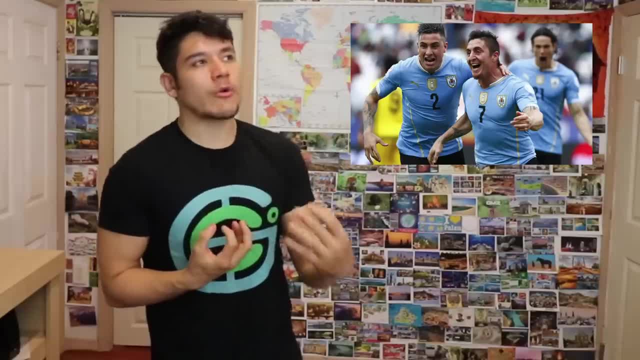 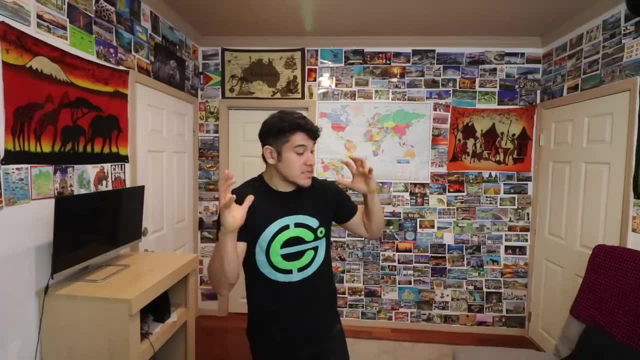 That eat as much grass as they can. Now, of course, you cannot talk about Uruguay without mentioning soccer football. Now here's the thing: Like all Latin American countries, pretty much love soccer football, But Uruguay it's like. it's impressive how well they've done for such a small country. 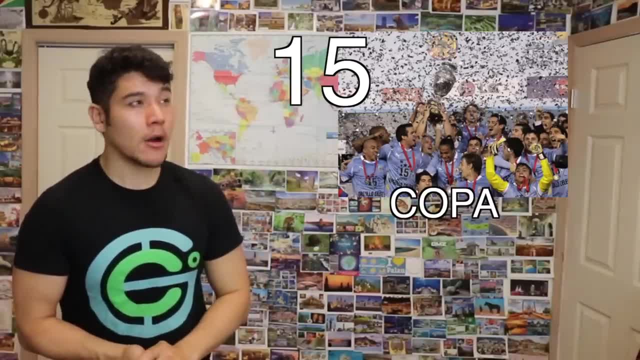 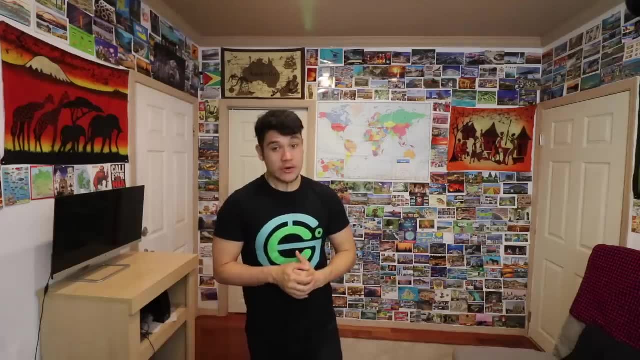 Nonetheless, they have won two World Cups and 15 Copa America wins. They beat Argentina, a country that's like 15 times their population, So they take this sport really seriously. Uruguay- What do you guys think? What comes to mind? 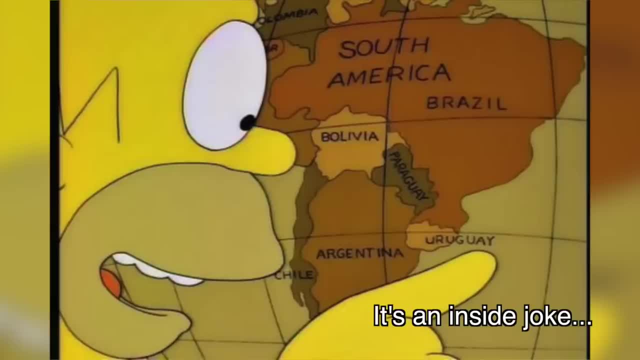 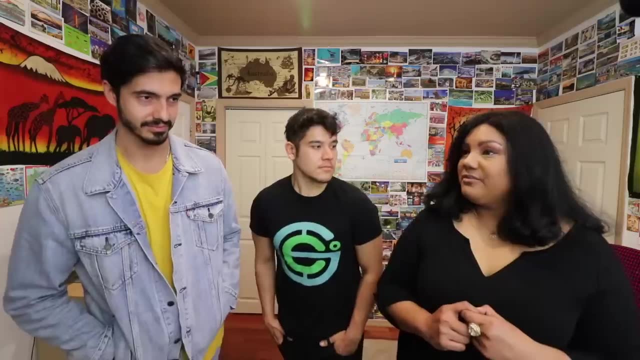 They seem so sure Soccer I can't. Oh, I don't think I've ever met a Uruguayan, but I mean they're cool. I mean you know I'll be cool with them. obviously They have, like, a very famous lake also. 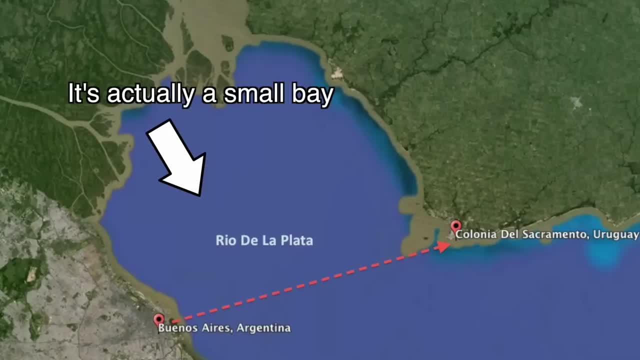 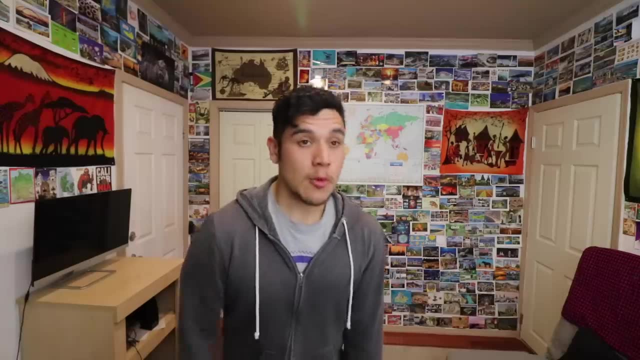 Lake, Lake, Yeah, Because everybody that goes to Argentina they always want to take like the boat ride. Yeah, yeah, I've heard that. And finally, Venezuela, Hey guys. so just a heads up: While we were filming this video, all those crazy things that were happening in Venezuela. 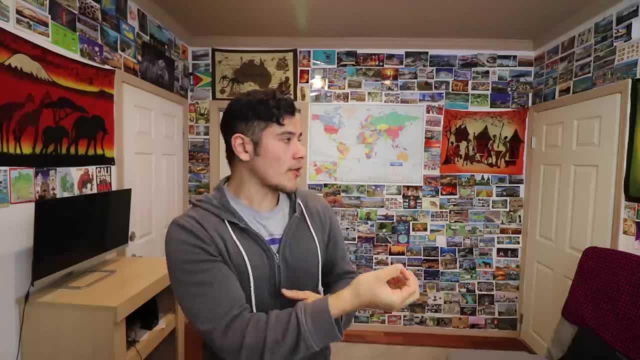 literally just occurred. So we're going to do a little video explaining about all that stuff later, But until then let's get back to the main video. Geograpeep Adrian says it might be boring. Geograpeep Adrian says it might be boring. 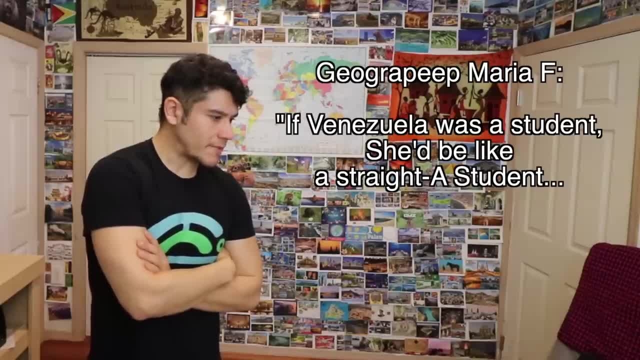 Geograpeep Adrian says it might be boring. Geograpeep Maria Fernanda says if Venezuela was a student, she would be like a straight, A student that got addicted to Adderall and is in and out of rehab. Okay, okay, jokes aside, 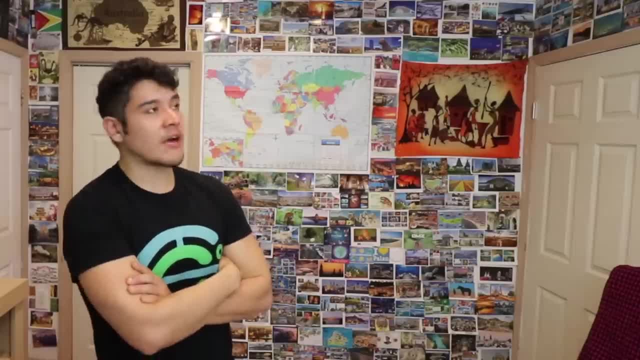 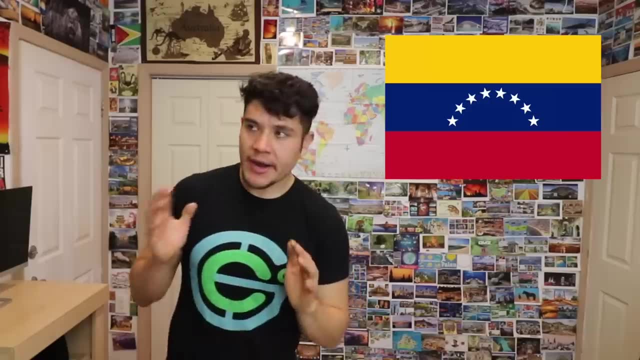 Venezuela is actually very unique. Just like their neighbors, they have almost every single landscape you can imagine: They have deserts, they have beaches, they have jungles, they have snow-capped mountains. Now, I know we're not going to talk too much about politics, but I think it's very interesting. 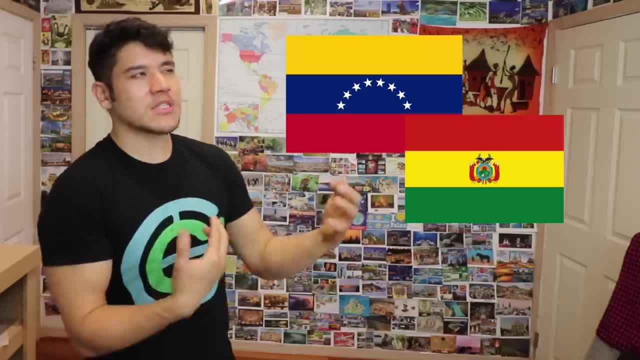 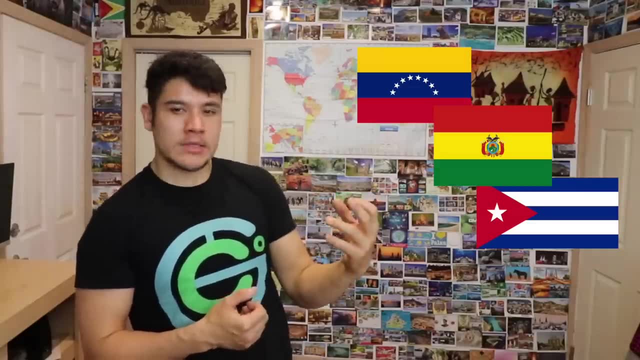 to note the relationship they have with Bolivia. Their governments kind of have similar ideologies, with like minimizing outside influence. there's like a unique Bolivia-Venezuela-Cuba alliance, There's like all these little hidden gems in Venezuela. You know, Angel Falls is here. it's the thing that inspired the movie Up. 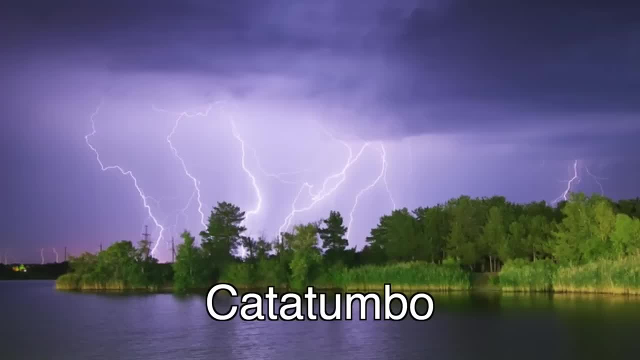 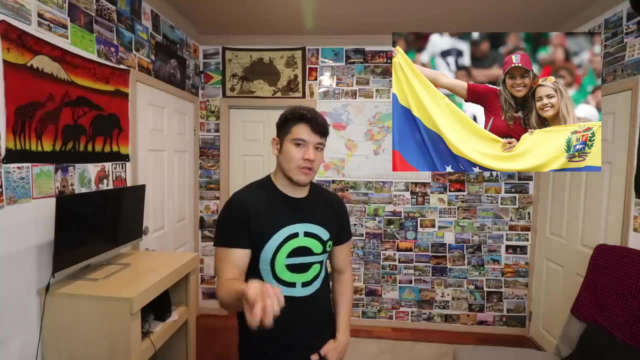 They have like a river, slash lake where it has like perpetual lightning all year round. And yeah, Venezuelans though, they are super proud of their country And Venezuelans do have a lot of European background. It's been said that Venezuelans have like the cleanest Spanish. 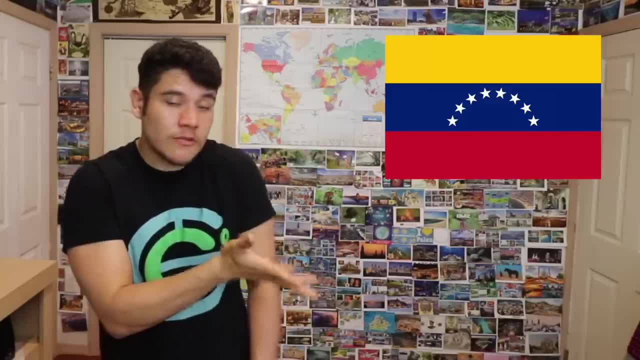 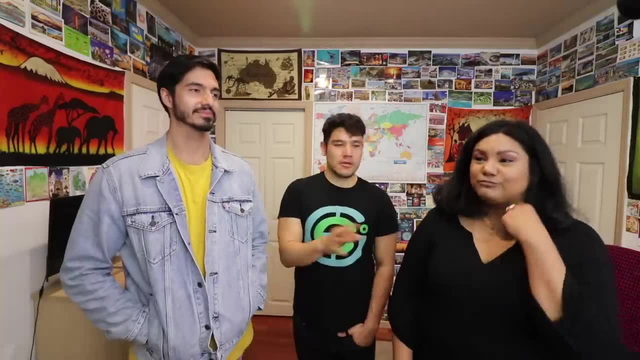 It's like very pure and untainted. I don't know. that's what I was told. They're very similar. They're very similar to Colombians, very outgoing and party people, if they want to be, Apart from all the political stuff. we all know it. but when you just meet a Venezuelan, 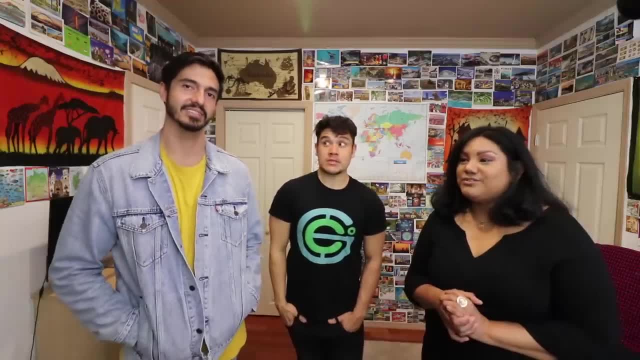 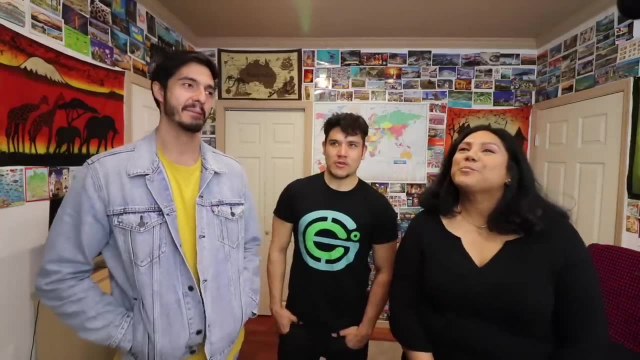 what do you think? The brothers, The brothers, The twins of you guys, Arepas? Uh-huh, Arepas, I didn't know. you said that, Arepas. No, you know the truth, you know. By the way, yeah, they do have a little bit of an accent. 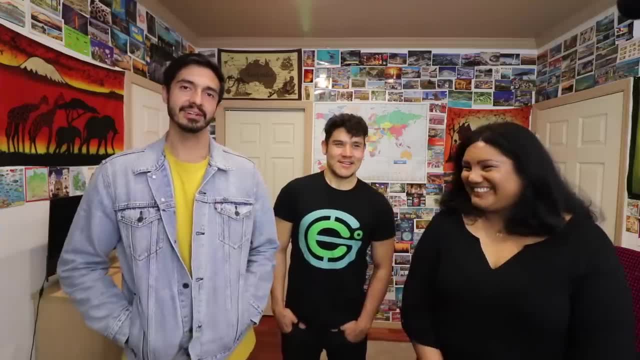 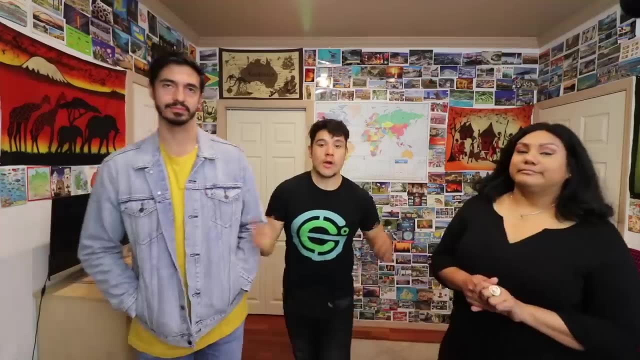 Diego, can you do the accent? Well, I can try. What's up, man? How's it going? All good, Nailed it, Nailed it. Oh, okay, By the way, Arepas Colombians. All right, and that was it. 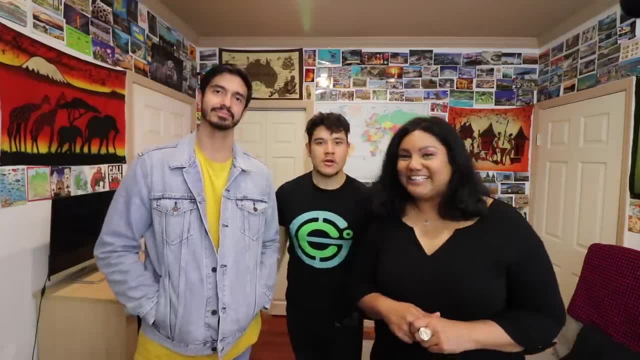 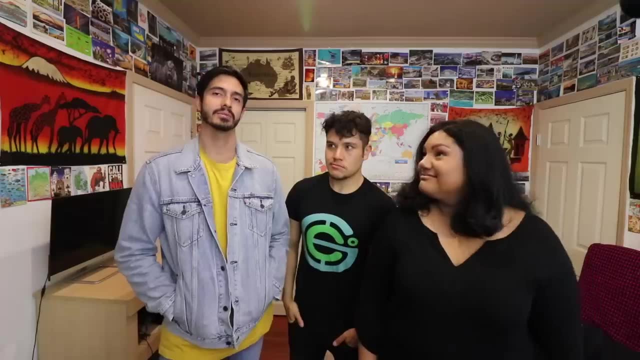 Thank you guys for being in this video. Thanks for inviting us. Yes, for sure, Thanks for inviting us. Any last words you guys want to just say to the whole Geography Now community: Even though we have a lot of differences, we share a lot of similarities as well, and 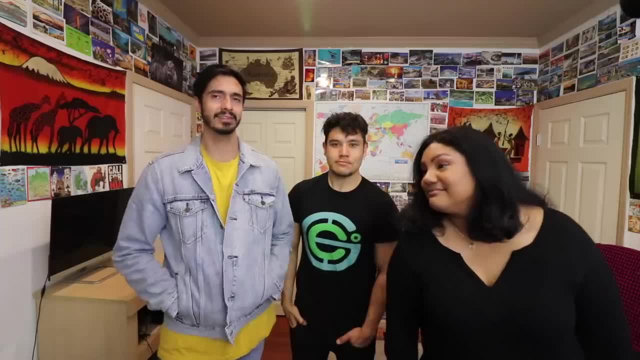 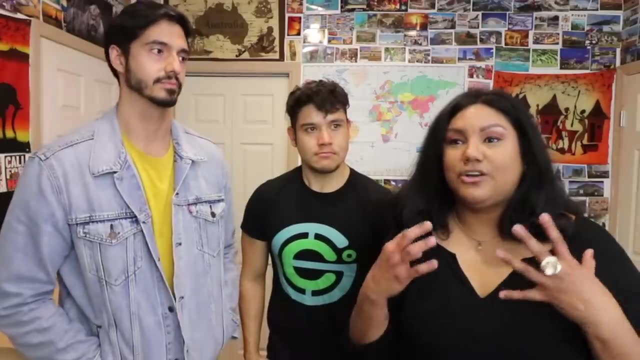 you will find really good people, really good food. landscapes are some of the best ones you could ever find. Yeah, I've had the opportunity to travel. It's just the nature. the colors are so vibrant. I feel like the Andes. 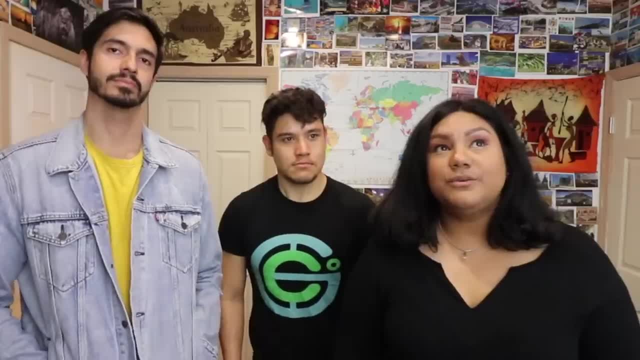 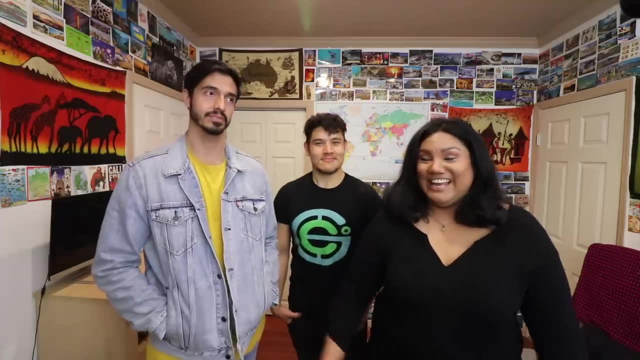 The minerals that we have is everything is just so organic and anything is like processed. Maybe that's the reason why the food is also so good. You don't have to fight for organic. You don't have to fight for organic. Everything is organic. 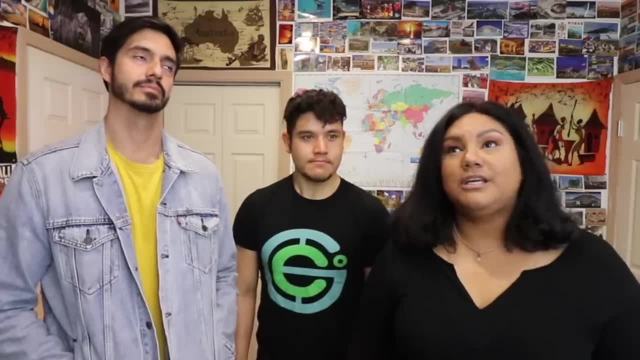 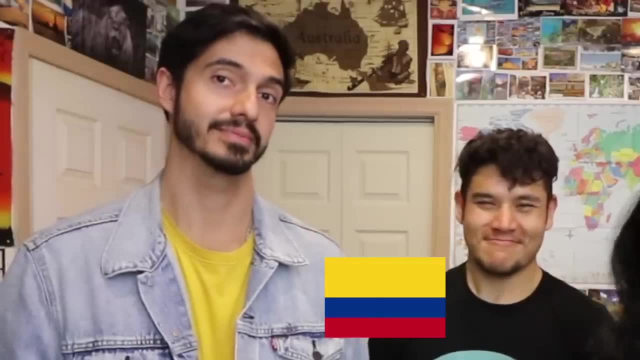 It's cheap too, right? Exactly, Every country has its beauty and you should visit them all. I will say Specifically which one should they visit: Colombia? Well, thank you so much. That's it. Hope you guys have a good one. 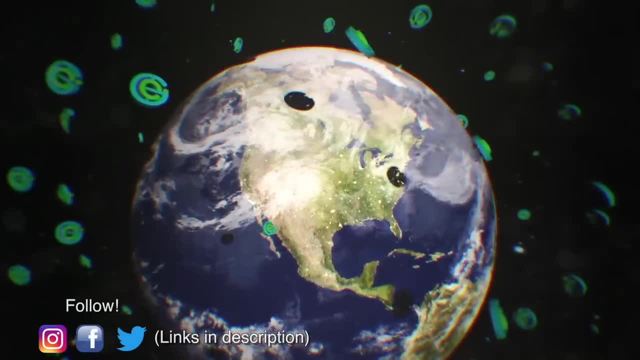 Bye, Take care guys, Bye, Bye. 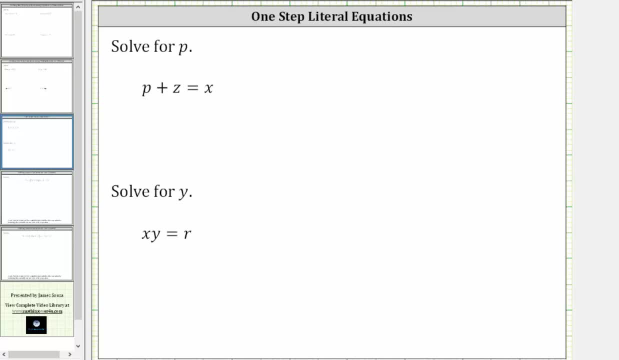 We want to solve each equation for the indicated variable. We first want to solve: p plus z equals x for the variable p. This means we need to isolate p on one side of the equation. Notice: right now we have p plus z on the left side.